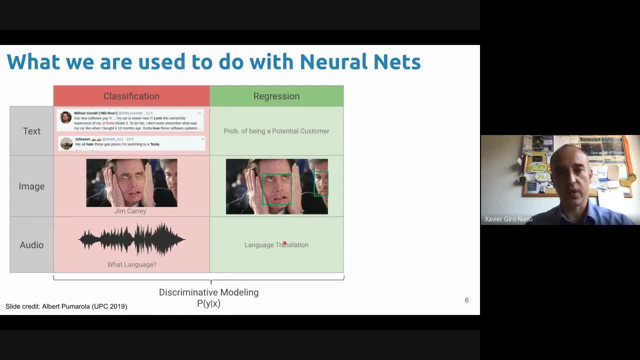 regression task that we can address, Or if we are trying to go from one language to another. we could think that that's a regression task, although I guess we can discuss a bit on this. But today what's important? It's today, we want to generate data, we want to generate new data. 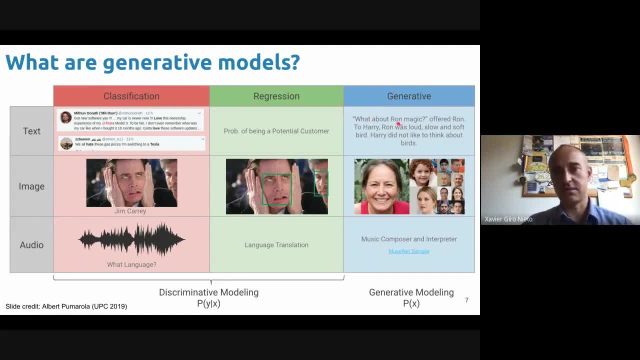 So we want to write checks. that looks realistic or at least that it's useful. Okay, so this text that you see here, it's kind of generated and it's supposed to be kind of related about Harry Potter books, or at least there's a word Harry, there's. 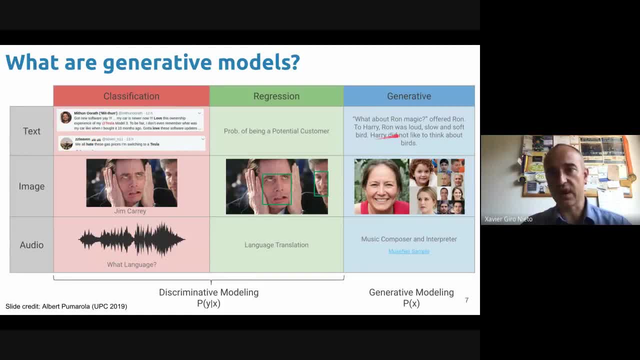 a word, Ron. what about Ron magic? or for Ron Harry, Ron was a loud, slow and soft bird. I don't like to think about birds, So it's a weird statement, but because it's basically generated by a machine and maybe 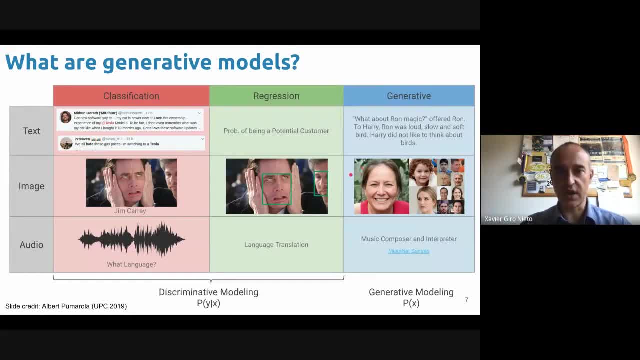 this point doesn't make much sense. Also, there are like images we can generate. they look very realistic, but they are. these people do not exist. Or we can even just use these models to generate new music, to compose and interpret new music. 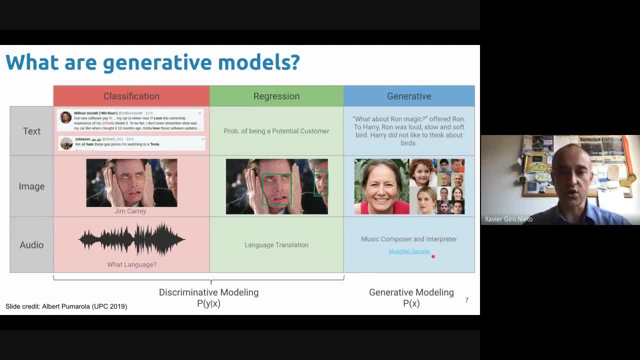 you can click here for a sample of it. So that's what we're going to be focused on, on generative modeling. So in the past, Basically what we tried to do is to predict labels out of data, but now that's not what. 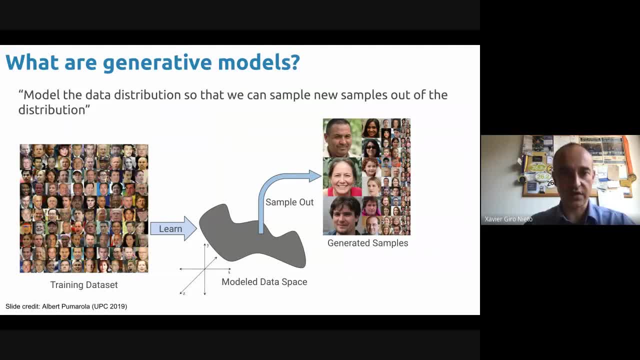 we want. What we want now is to model the distribution of data So we can sample new samples out of it. There's still going to be a training data set. we still need some data to train our model. We'll take our training data set. imagine we have a large training data set of faces. 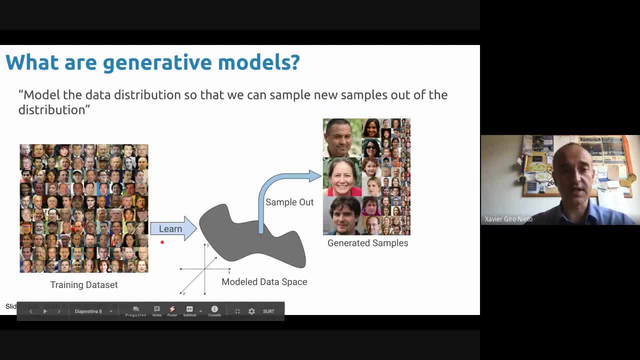 of people And from that Training data set. what we would like to do is to learn some distribution, data distribution or some manifold in the data space so that, if we have it properly defined, we can generate new samples out of it. 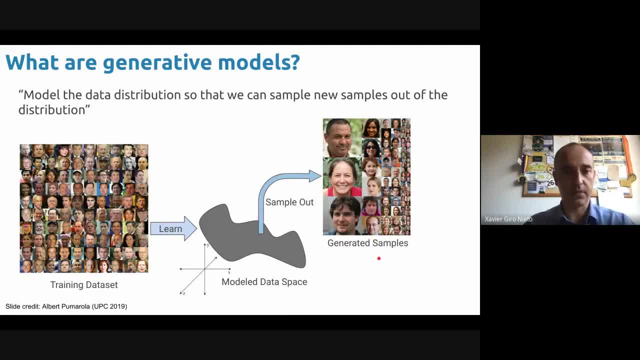 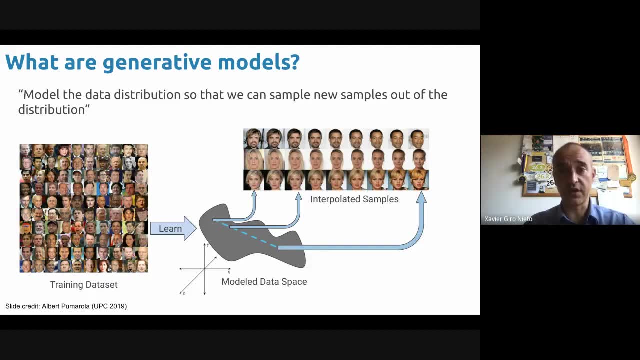 We can generate these kind of faces of people that do not exist. Not only that, not only can we generate new samples, but we will also be able to interpolate from one sample to another. For example, Here you see how you can move from one face of a famous character into another one. 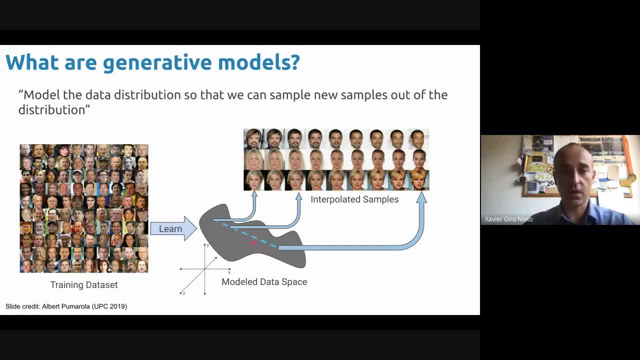 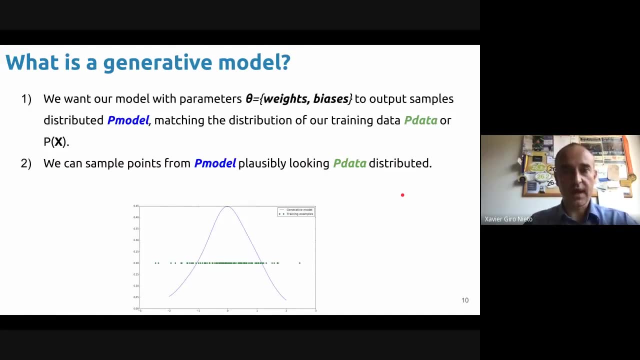 And that's because in this data space we'll be learning, we'll be able to, let's see, interpolate, to generate samples between any two points of this space we are learning. Okay, So you can see here all the evolutions In a less fancy but maybe more clear way. here you see what we'll be trying to do. 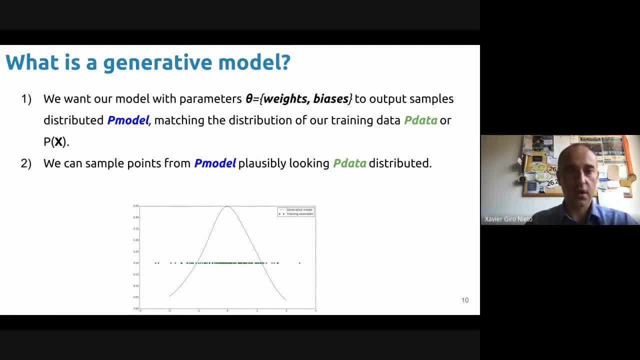 We'll still be trying to model our network with some parameters. in our case they are going to be weights, they are going to be biases And we are going to, based on these weights and biases, to go to model the data of our 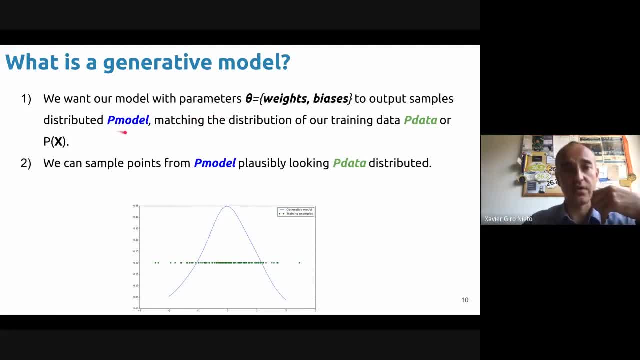 model, hoping that the probability of distribution of data of our model will match the distribution of our training data, that sometimes we will refer to it as p of data or p of data. If you can do that, later we'll be able to sample new ones. 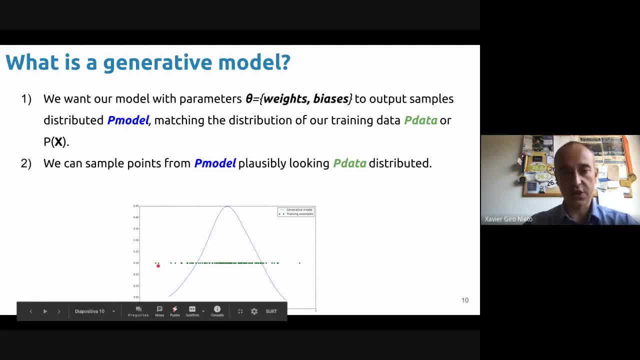 For example, imagine that we have this, this toy example, in which our training examples are the samples in green. As you can see the samples in green, they seem to follow a Gaussian distribution, in the sense that most of the samples are in the center, not that many in the skews. 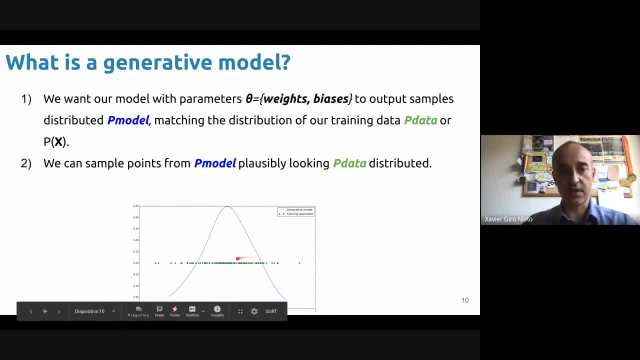 So by looking at this data, it will be possible to estimate the mean, the standard deviation and the error, And with these parameters we could predict the distribution, the distribution, and if we have the mean and the standard deviation, we can also generate new samples that follow: 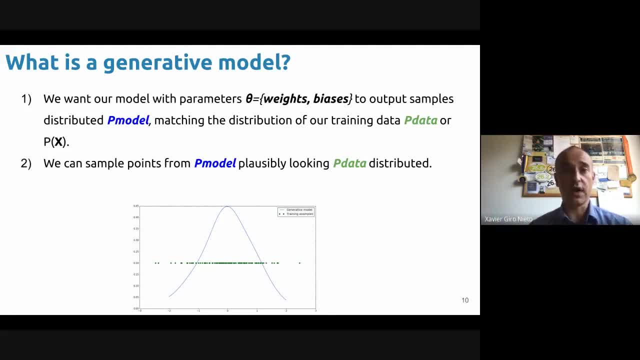 in this case a Gaussian distribution. However, in our case we'll be not be assuming that we have a Gaussian distribution. We have a neural network that can approximate any function or at least as a field right, Or at least very complicated functions, much more complicated functions. 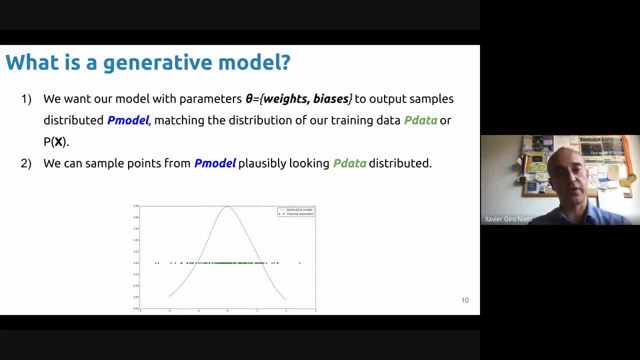 We can do that, we'll be able to generate very realistic data. Again, let me insist: this is not about an architecture, so don't expect a recurrent layer or a graph neural network as Javi presented in the previous lecture. This is just a concept of how, what our generative model is and in particular today with GANs. 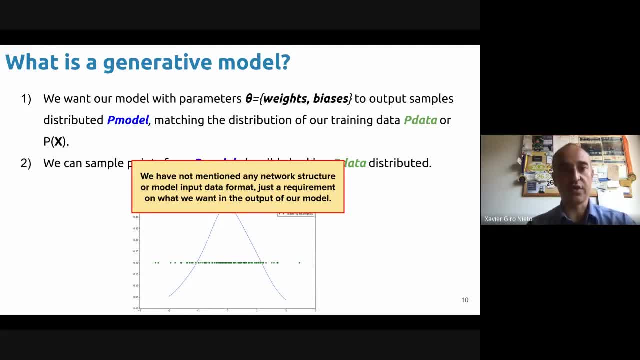 I will not really focus a lot on any of this. And in architecture, you see that most of my examples they are based on convolutional networks because we'll be dealing with images, but that doesn't mean that you need to use convolutional networks to generate data. 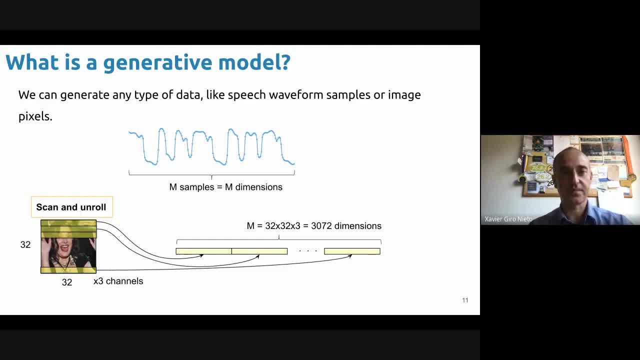 You can, for example, use these graph neural networks that Javi mentioned. So, once we have that, if we are able to generate, distribute, to model our data distribution, be able to generate samples of any dimension. so, for example, imagine that we want to generate. 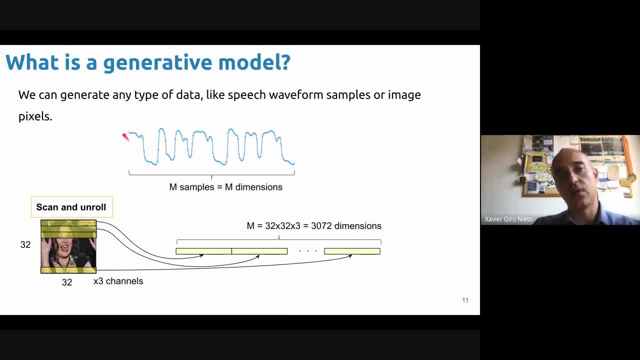 speech. You can think that now, with our speech signals, they are placed, located in some space of n dimensions. You can think about that. Or what about images? You can think that images, if you just read them, pixel by pixel, in this case, we'd like. 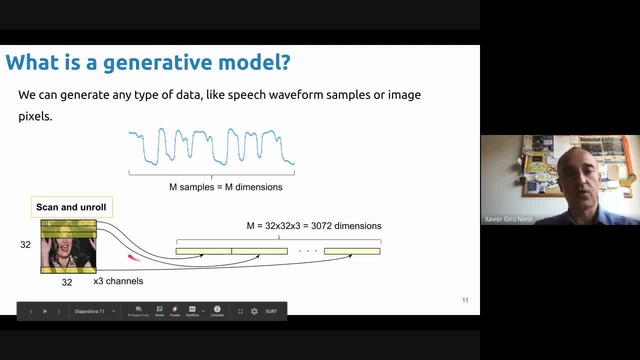 32 pixels and three channels. you can. you could just put them all together, just one x for another, just flatten it and then unroll it, and then you can consider that an image is not more than a point in a graph. 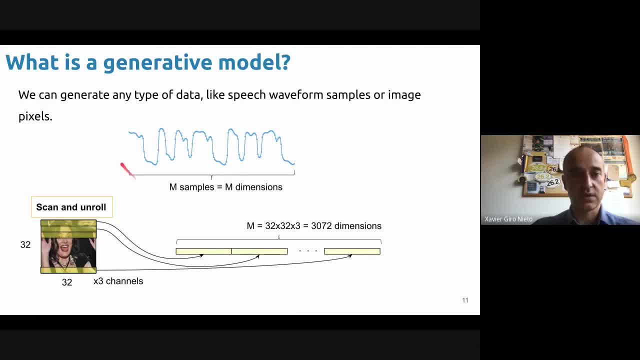 It's a point in a high dimensional space, okay. So, whether it's speech or image or any data, you can in the end think, imagine that it's a point in a high dimensional space and in that high dimensional space we can try to. 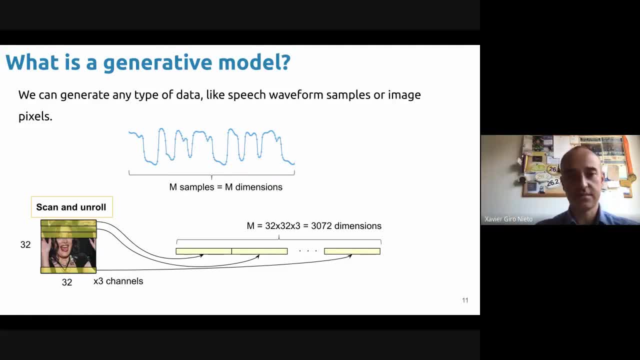 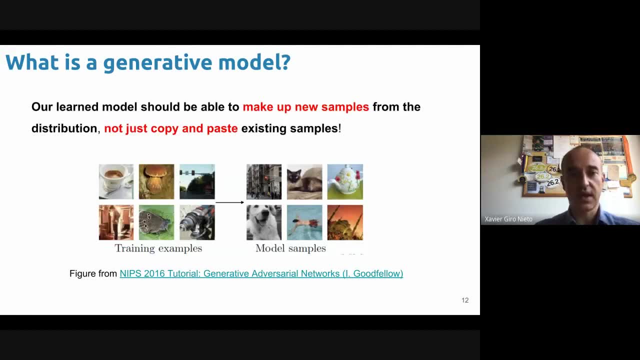 estimate the distribution of the data. If we do that, we'll be able to generate new samples from our data distribution, our approximator Notice. What we want to do is to generate samples that they were not in the training data set. We are not again. as in discriminative tasks, we don't want to memorize our training data. 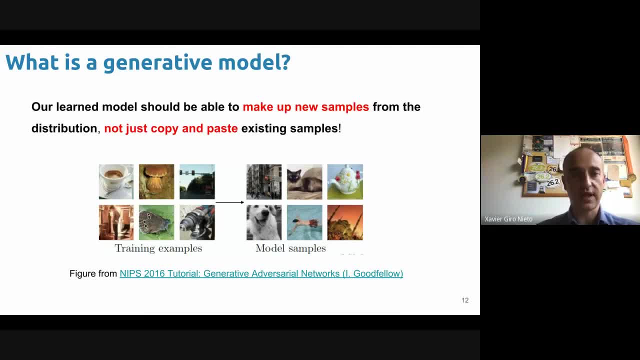 What we want to do is to learn some parameters that will allow to generalize well, So, in this way, to be able to generate new data that look realistic. The example you have, these training examples that were used to train a neural network that later may be used to generate new samples like this one. 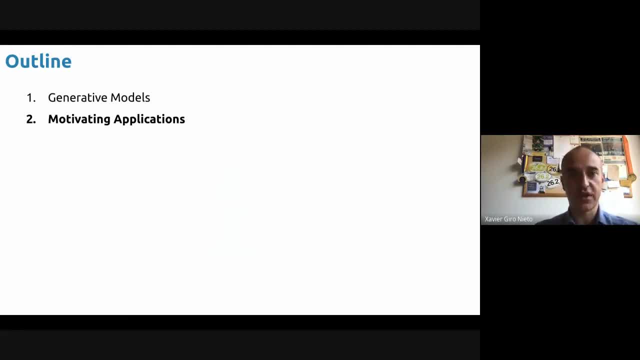 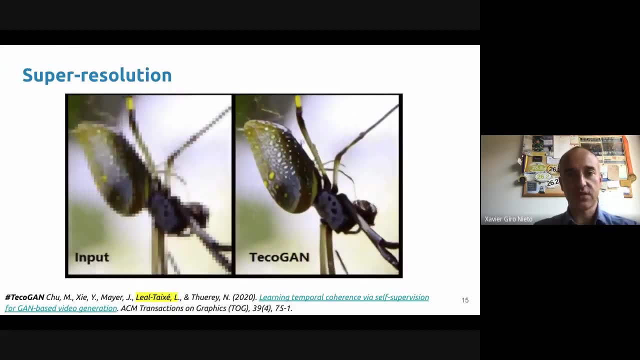 Let's look at some motivating applications so that you see what I'm talking about. One application could be like super resolution. I guess that's not this work in particular, but one of the other work. previous work that kind of showed the interest in terms of GANs for applications was super resolution. 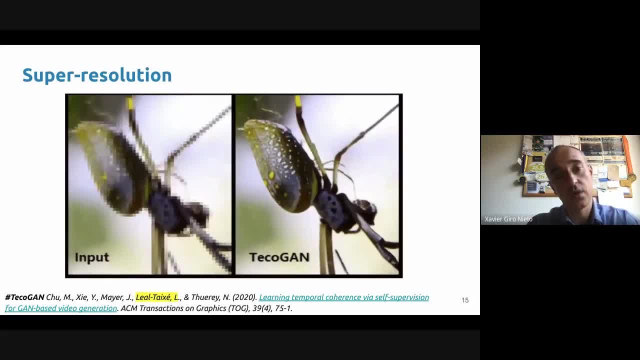 Imagine you have an image or a video in low spatial resolution. That's what you have in the input on the left And on the right You have the output of a GAN-based model that has interpolated, let's say, the missing pixels in a much better way than just what the linear interpolation would do. right, 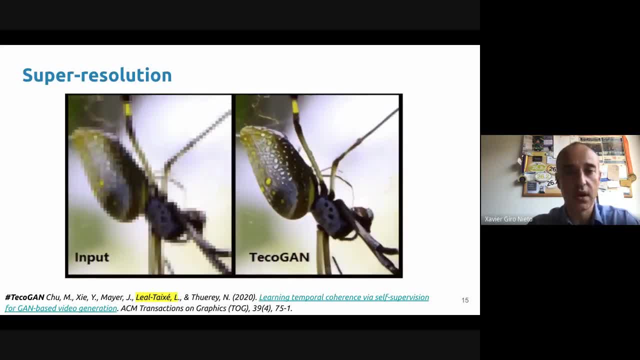 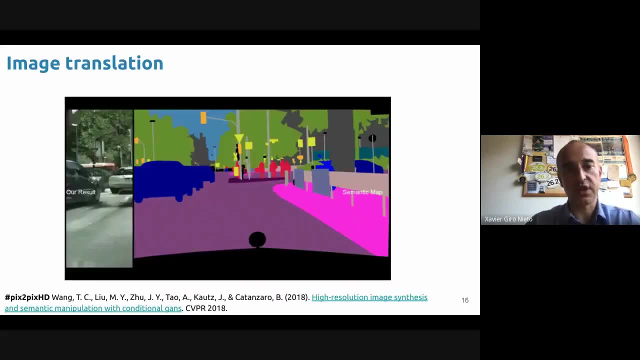 There's a lot of detail that has been added and it's based on a previous learning process that the model did. This work actually was co-authored by Laura Leal, who was a former student from our university at UPC. It's not a very 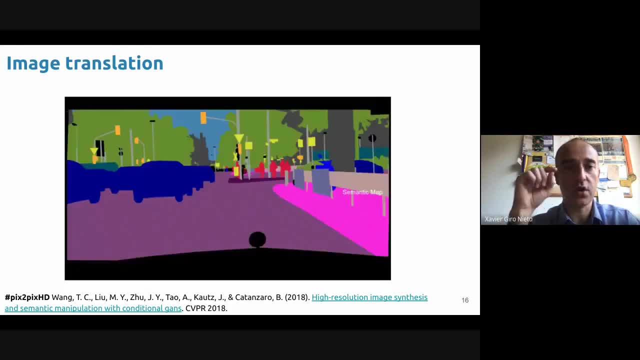 That's the first image that you see. that's called a semantic map, So each color corresponds to a class. For example, the blue color corresponds to the class car. You can feed that into a GAN so that it's going to generate a realistic view of a scene. 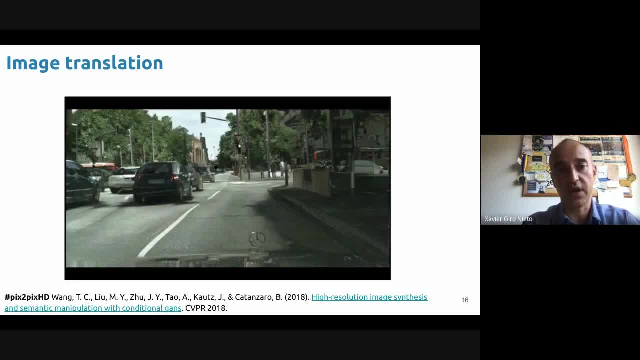 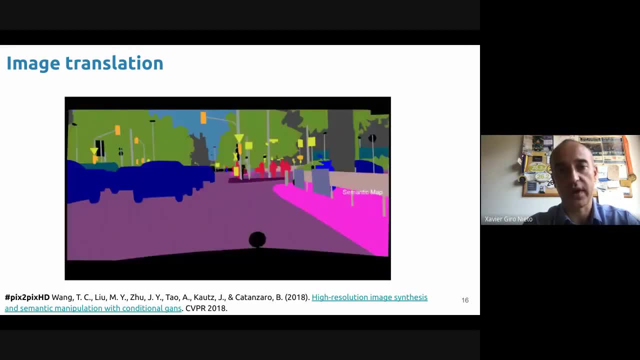 that matches the pixel labeling that we can generate. So that's a way, for example, to generate a graph. And then, of course, the second thing is that the GAN is not just a graph. new training data. If you have a simulator, you don't need to have a very super high resolution. 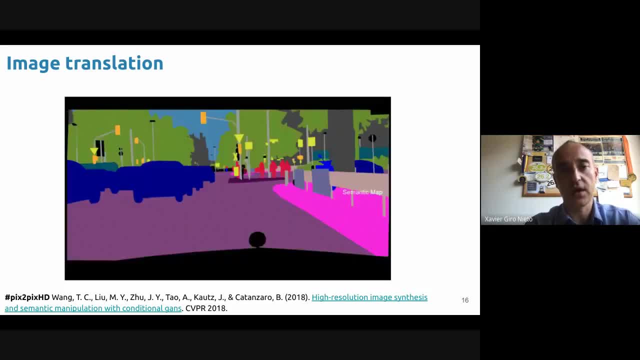 simulator. As long as it's doing the physics part, you can have a simulator for autonomous driving, generate a large amount of data, even if it's as simple as this as this child, and then have a diamond shop that will actually produce a visually realistic. 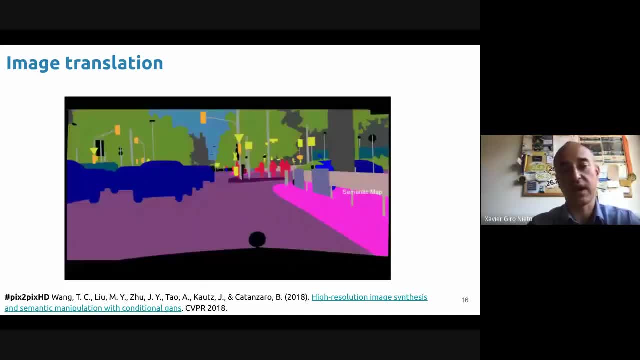 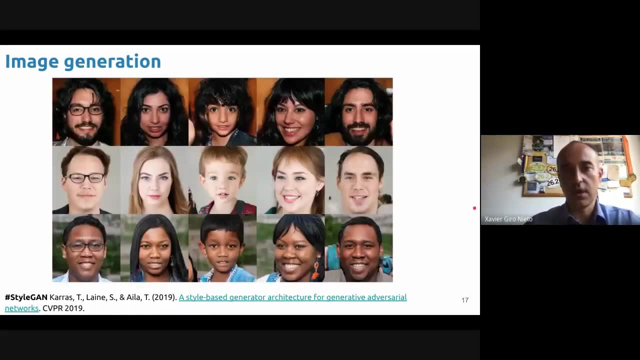 output of the video sequence And again we can have a lot of data for training our neural networks. This is one of the, also following on the idea of generating faces. That's a more recent work called StyleGAN, in which they managed to, let's say, transfer styles between, this case of faces, or 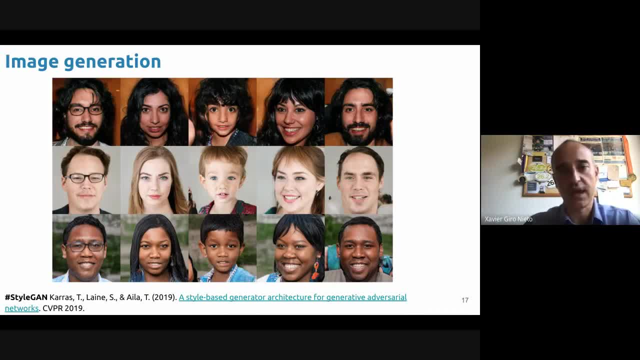 there are also like examples with animals or stuff, as you can see. So in the first column they are all generated synthetic faces. Okay, so they are always a male person wearing glasses, second one, a female person wearing glasses, third row child also like a similar pose and in face expression, So we can transfer. 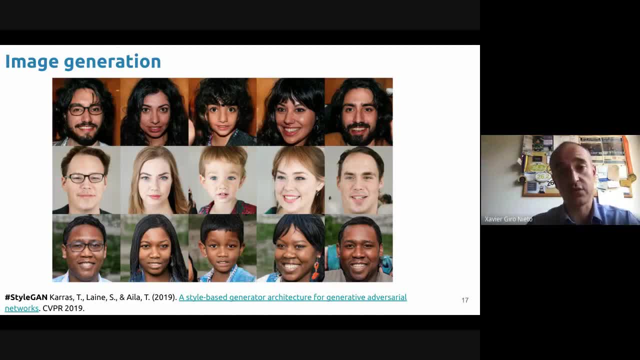 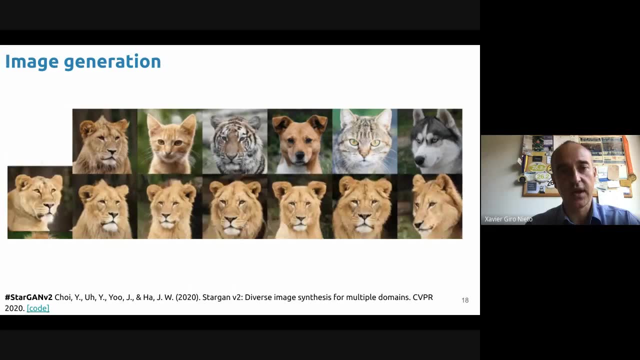 actually attributes, facial attributes or skin attributes across different synthetic faces. Okay, totally generated. Okay, that's the example of the animals I had in mind. That's one of our work as StyleGAN. It's kind of a similar approach, more recent, As you can see. 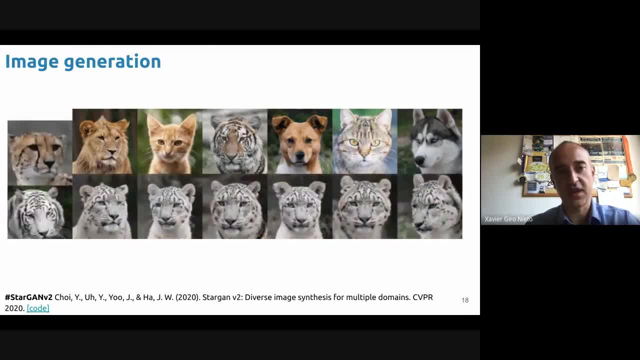 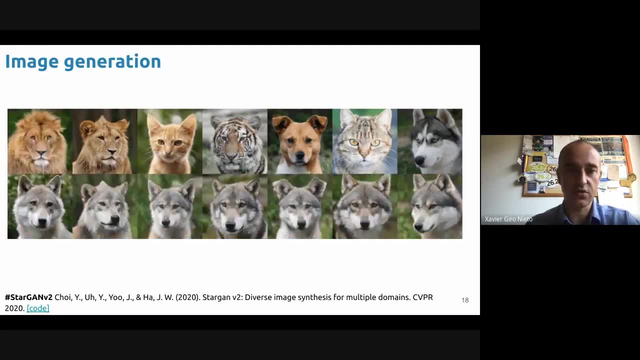 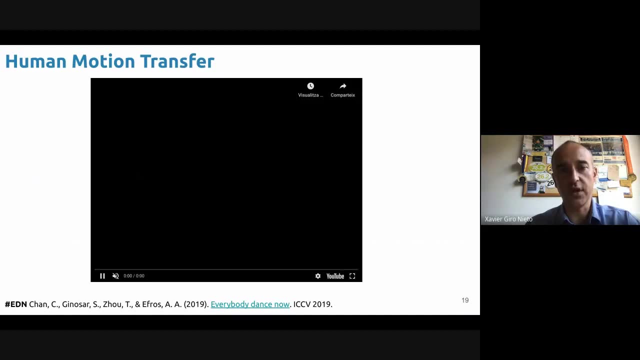 you can. it doesn't limit only to faces Here you can. they use it for a broad amount of domains. I mean, in this case, that's animals, right, But all these images that you see generated, they don't exist in reality. What about if we go to video? 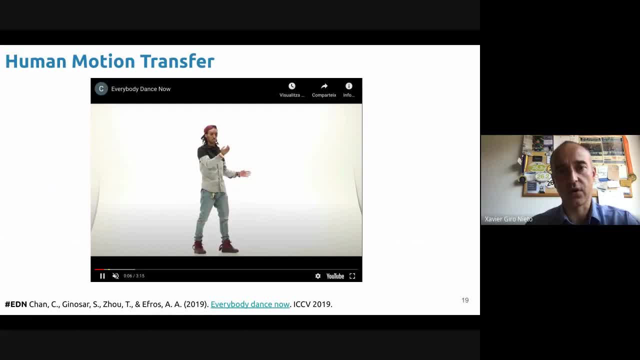 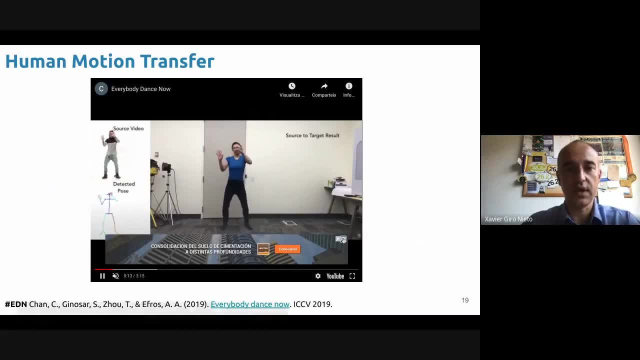 In this work. imagine you have a source subject that's being recorded doing some motion, and then a target subject that you collect a training dataset And then after that, what you're going to do is you have the source video here on the top left over here. 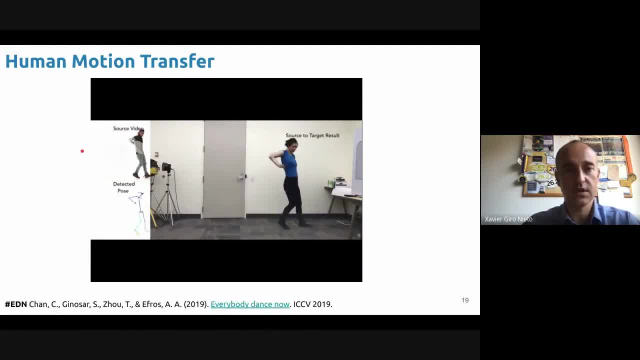 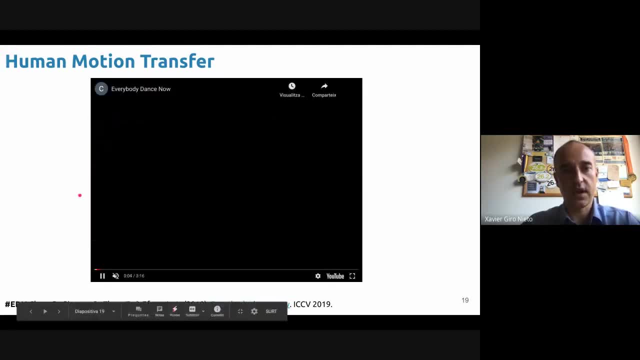 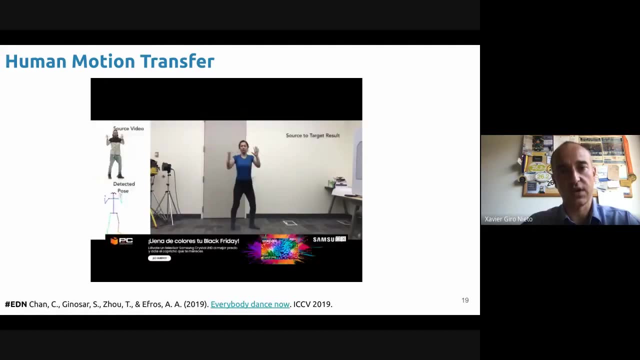 So this here? okay, that also doesn't move, but it's this server here And the lady in blue that was automatically generated. I will start again Here. you have again the source subject and this motion is transferred to this lady. it's a training dataset, Okay, And now what you see. 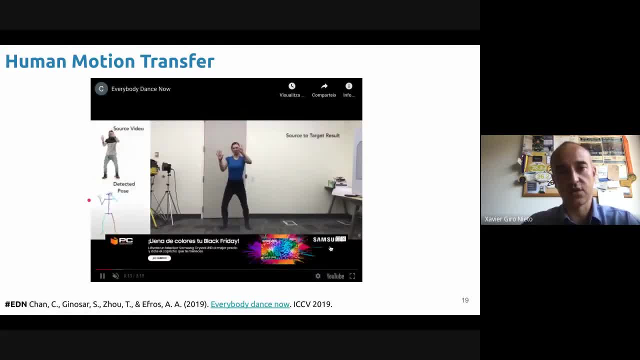 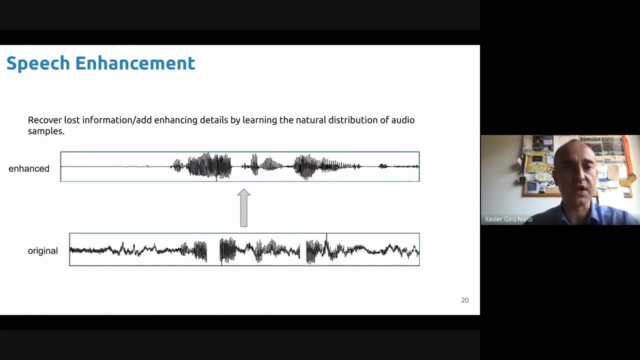 the big screen is a source to target result. Okay, In this case they went through the detection of the pose And later I'll show you like another application that we developed at UBC based on this algorithm. Another interesting application would be like for speech enhancement In many 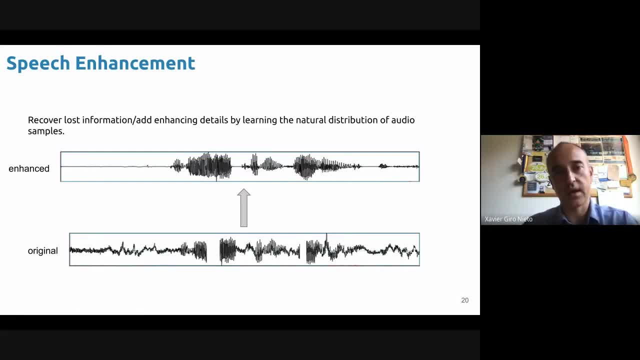 situations, the spoken words, they suffer distortion. Maybe there's a cut in the communication, Maybe you were speaking on the phone at some point, There's some data packet loss at some point, or maybe you are in a concert or recording a studio and some part. 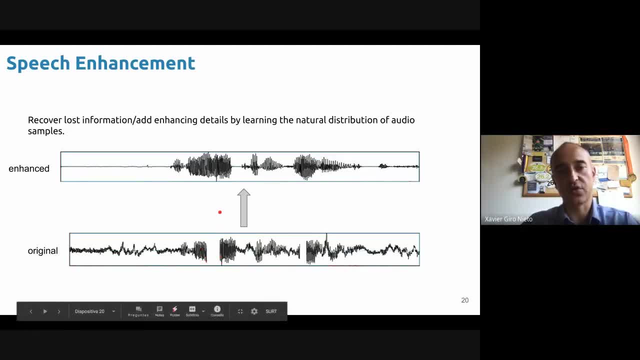 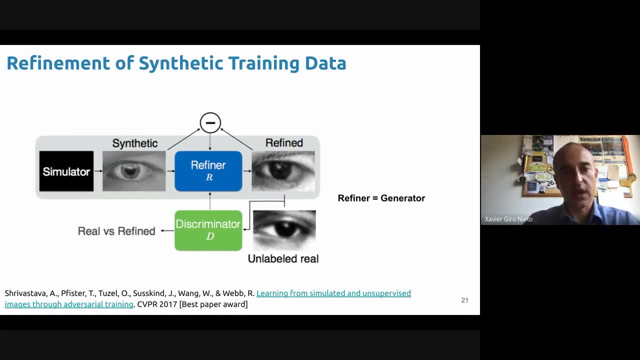 of the data was missing. It's possible to reconstruct or clean, to clean up the data with generative models. Okay, This would be one of the best paper awards in 2017 in CFBR, which actually they- that was what I mentioned earlier- that they use it. 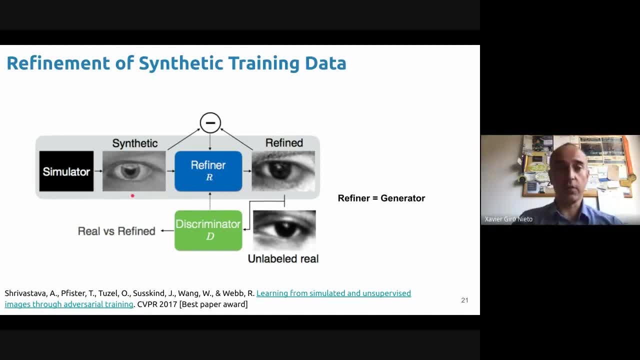 GANs to generate synthetic data. It's one of the few papers from like Apple. What they did is they wanted to have a large dataset for eyes. As you can see, this eye is synthetic. If you notice, it looks synthetic when they use it as a GAN, just to refine the synthetic. 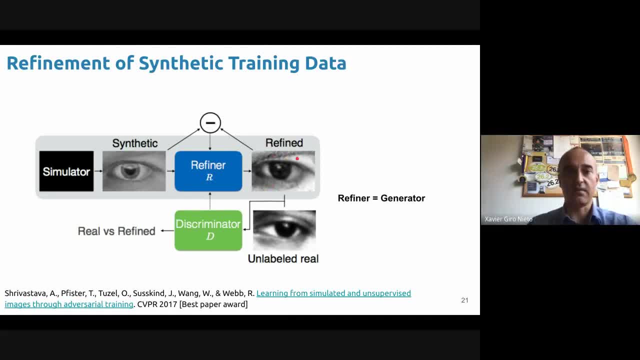 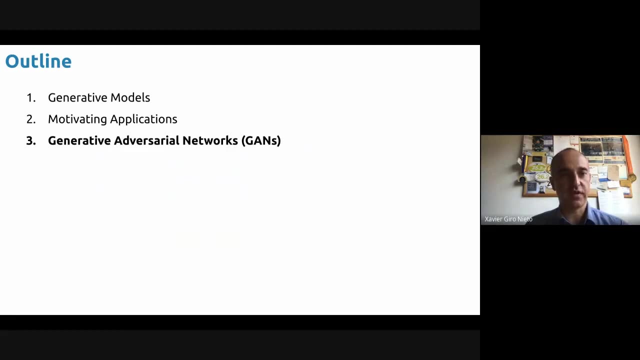 data. So this way they had much more training data- like as much training data as they wanted, because they could generate any eye gaze. they want it and then just refine it to make it realistic. Yeah, Any question about applications so far. If not, I'll move into explaining how this is done with Deep Neural Networks. 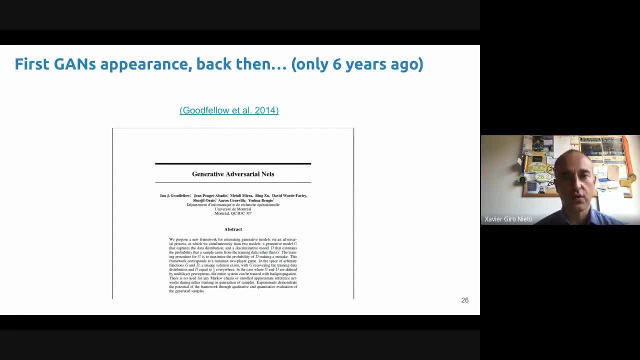 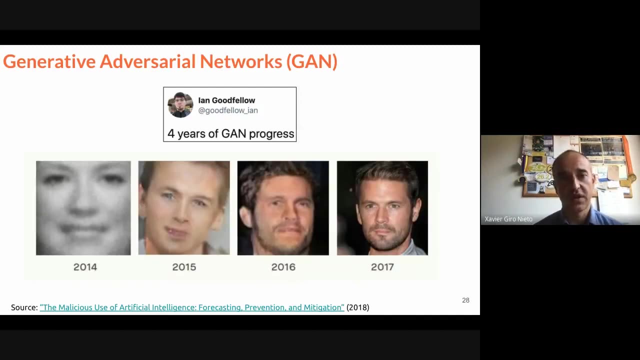 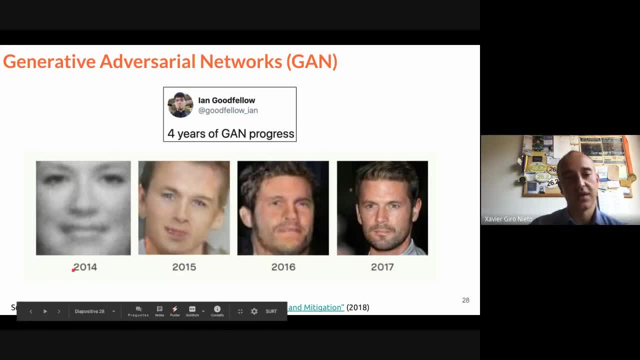 to check that. that's not only us, but I'm being familiar with people who are using these glasses, So this works quite well at Apple. I'm like: oh, my head bleep. Here comes the photo you gave us of Bruce broke it. 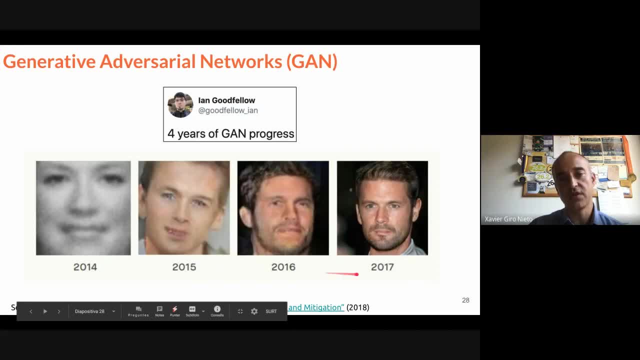 Ok, so right now I want you to show me how this would work back home. So, if you do have seus, like on the left, you can see the quality of the first sample of 2014.. That's the quality that face is being generated by GAN and these mehr than 40 years, 2017.. 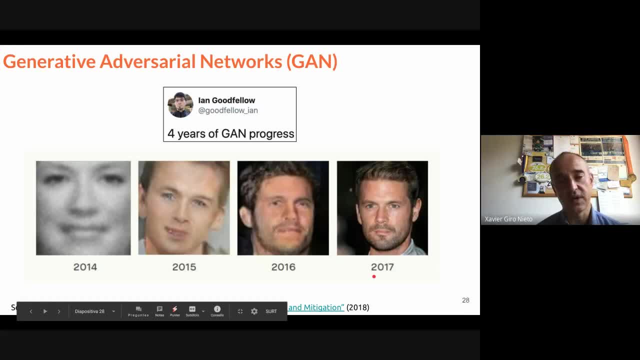 00 hunter in 20 and actually earlier. I show you like even more recent evolutions of of that, So, of that. So you can see that this field has evolved very quickly and that it will probably still evolve much faster in the future, because it's a very convenient way. 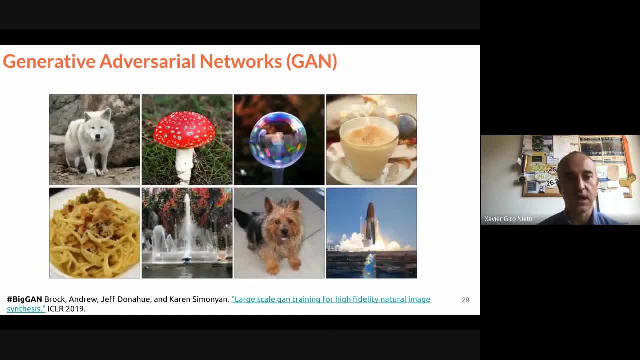 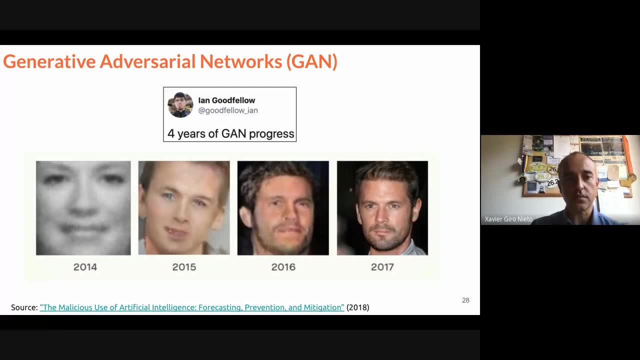 of generating data. This, for example- one of these examples that are well-known, that's called the BigGAN model- was presented last year in iClear, And you see that the quality of images is much better than what we had in 2014.. 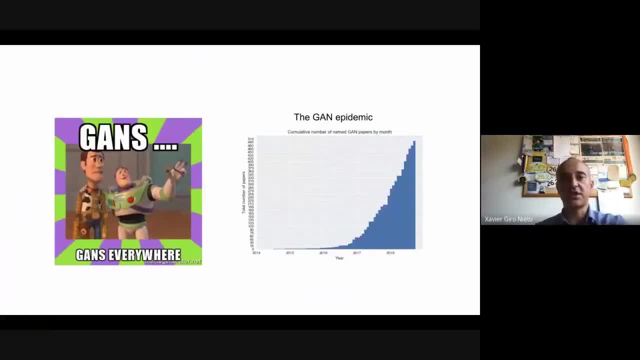 So since 2014, there has been, as this chart says, kind of a GAN epidemic. There are so many scientific works focused on GANs. Actually, now notice as well products like apps or software that is exploiting this technology for video manipulation, for content generation. 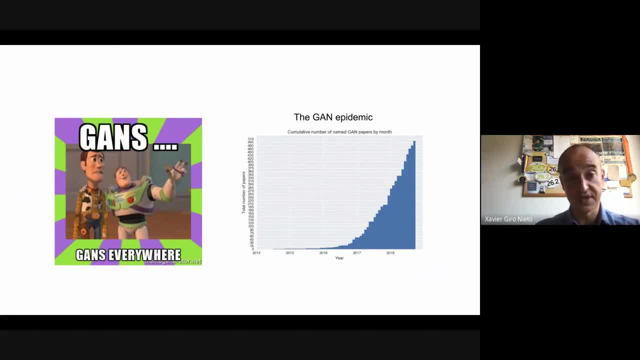 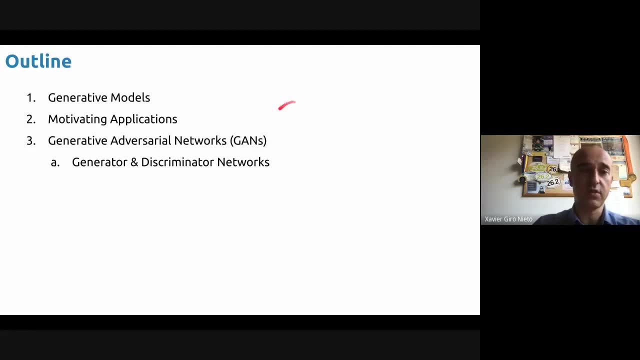 artistic creations And there are many opportunities for you. if you're interested, Let's see how it works. Genetic fibers have networks. As you notice, it talks about networks, So there will be not only one network, but two. So that's more or less what the image I 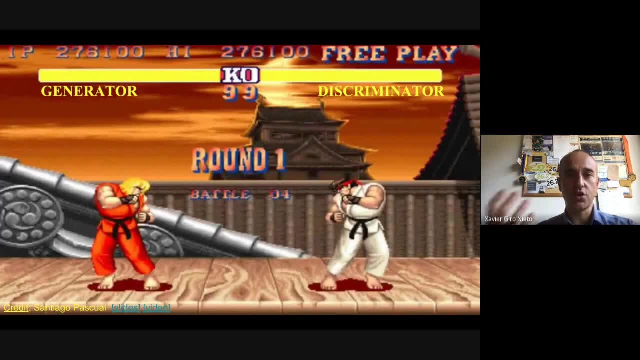 would like you to have of each. We'll be having two networks, One of them is the generator And another network is called the discriminator, And they will be kind of fighting each other And our goal, actually, as a data scientist. 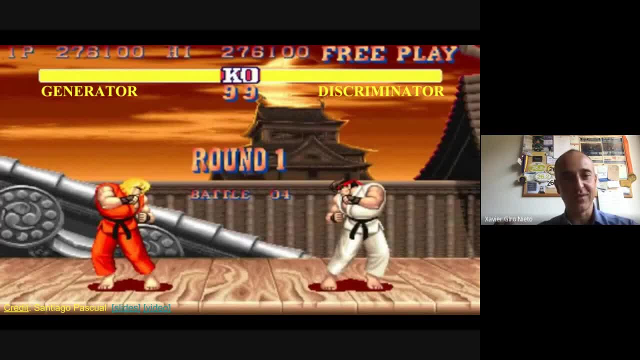 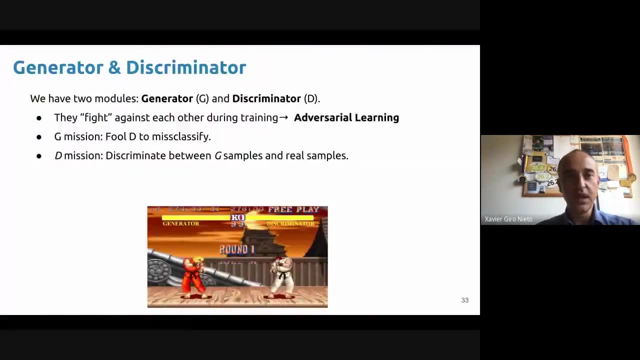 will be that none of them wins. Actually, we would like them to just keep fighting as much as possible, because the more they fight, the stronger they get and the better they get. So let's see exactly what are they fighting about. So when they are fighting, they are learning. 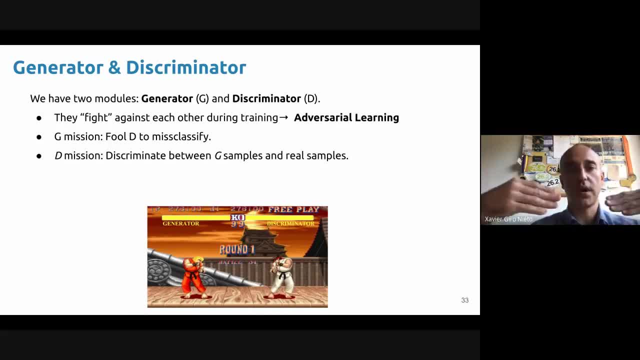 So it means that we will be estimating the parameters of two deep neural networks And they will have contrary goals to each of the networks. So when I talk about G, I will refer about the generator, And when I talk about G, I refer to the discriminator. 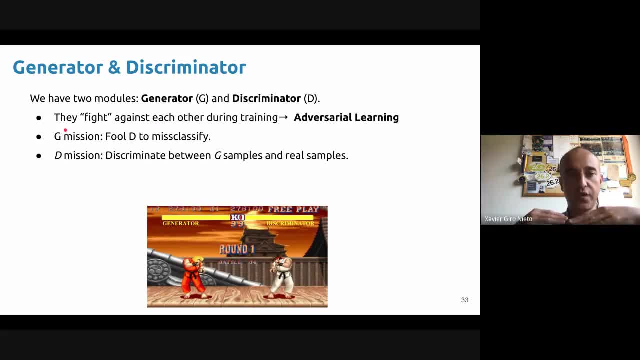 Then the mission for G, for the generator, will be to fool the discriminator, to cheat it. So the discriminator makes a mistake in a classification task. What is the classification task for the discriminator? The discriminator will need to decide whether a new data sample- let's put, for example, an image- 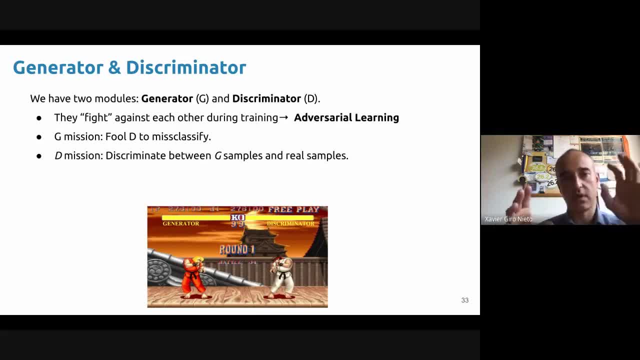 But again, it can be a text speech whatever. Let's say that you have a sample that was produced by the generator, So the generator is actually the one that produces the samples. So the discriminator will need to give a sample to decide if that sample was produced by the generator. 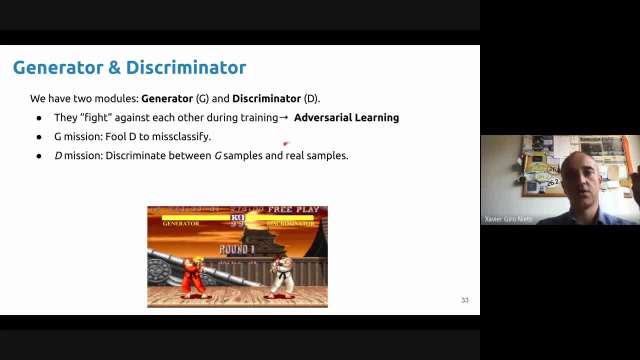 or if it came from a training data set. So remember that I mentioned that We still need a training data set. We still need real samples. Good news is that these samples do not need to be labeled. We just need them to be real. 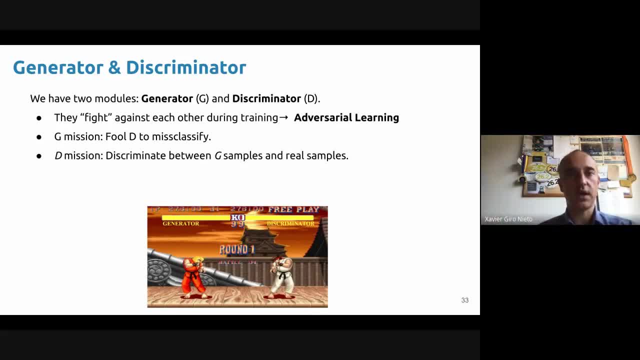 So we don't need annotators. Just collect data. Just take your camera, Start taking pictures from everywhere that you are interested in the domain And that's going to be your training data set. No need to label anything. So this contradictory goals the generator trying to mislead. 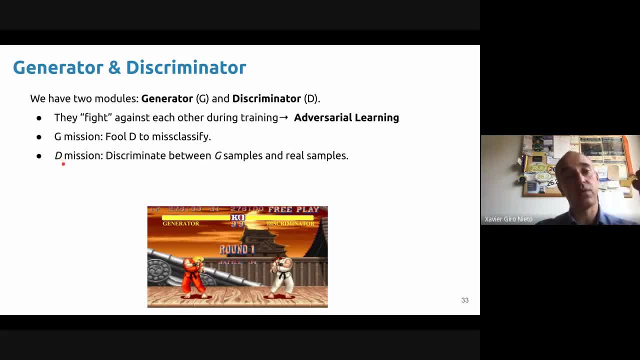 discriminator And the discriminator actually trying to figure out if a sample was produced by the generator or it was a real sample. If they both learn at the same pace, we will succeed into training generative adversarial network which, I warn you now, it's not a piece of cake. 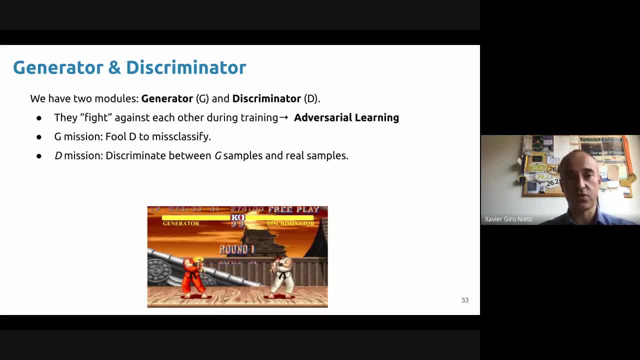 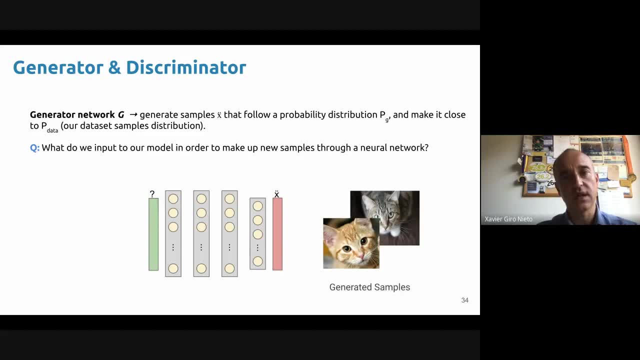 They are quite unstable in training. It's not easy to train these models. Let's look at it in more detail. So what the generator does? it's going to generate samples that will follow a protein distribution, which is the one that we want: to make it be as close as possible. 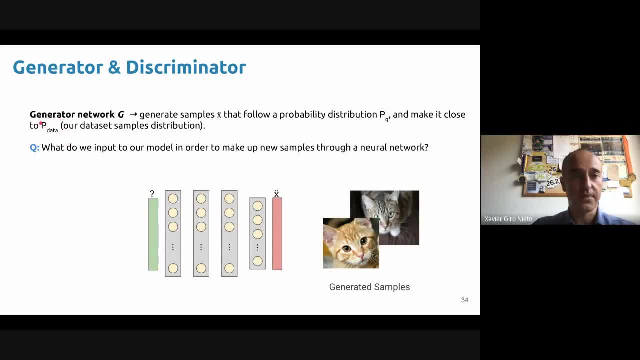 to the real data distribution. We call this p of data. That's going to be our training data set, Then. so we have a neural network that will be generating samples of the output. We like these samples to follow the same data distribution as the real one. 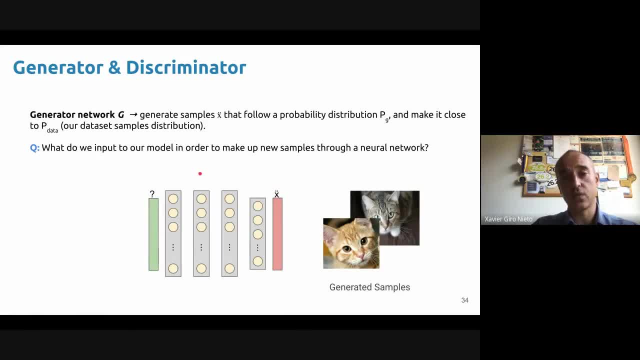 So if we want our data distribution to be the same, we want our network to generate cats. We would like the network to generate different cats, So the cats, but not always the same cat. We would like it to generate different cats. Then what could we do? like if we assume, 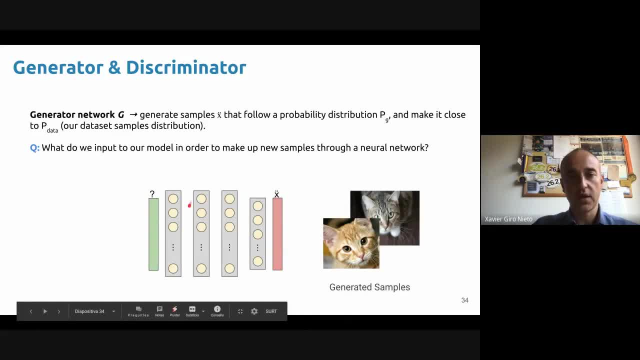 that we have our generator strain but that we would like to have different outputs if we can only change the input. Because here I should tell you that generator is a network. I talk about the output, but I didn't talk about the input. 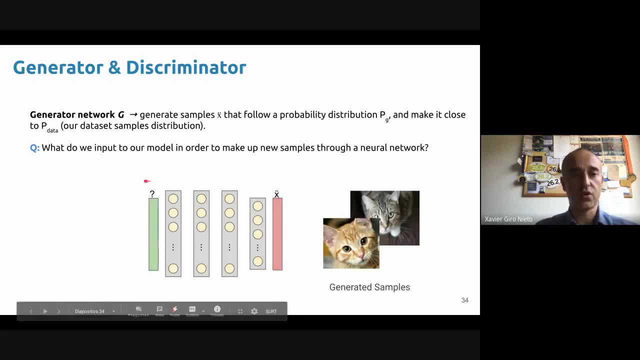 So what do you think we could use as an input, so that at the output we're going to have different, let's say, a diversity of generated samples. So what could be the input You can write in the chat If you all turn your microphone on, that's going to be recorded. So if you don't mind turning your microphone on, you can write in the chat. If you all turn your microphone on, that's going to be recorded. So if you don't mind turning your microphone on, you can write in the chat If you all turn your microphone on. 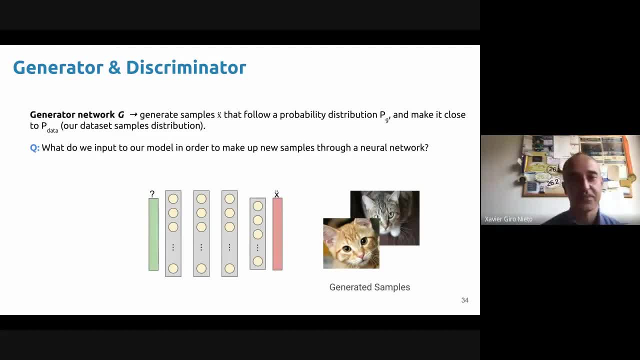 you can write in the chat, But that's an open question for you. So some ideas. We would like some stochasticity here. We don't want the network to always predict the same cat, because that's going to be very useless. So how could we have some stochasticity here? 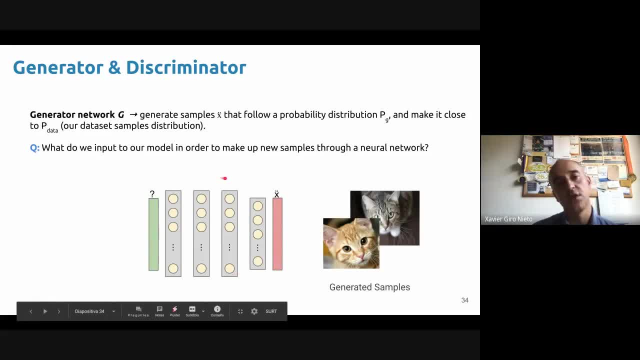 So introduce some force, some stochasticity into the network. So remember the network is in the end it's just a set of weights and biases connected with the neurons, whatever convolutional or whatever neurons. But so far what you have seen in the course is that when you feed some input sample in a network, 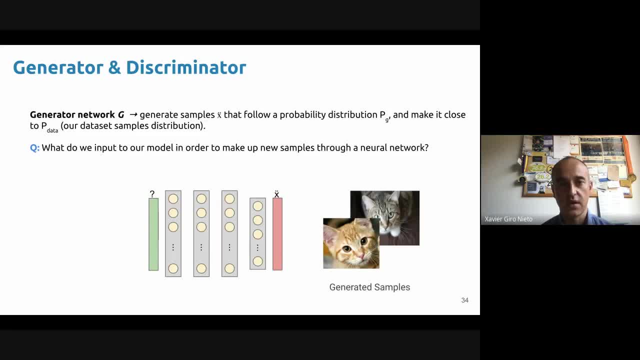 once and again and again, the output is always the same right? So when you train your network with MNIST and you show a digit- number two- and you feed that image of number two and then number two and you feed it again, you'll get again number two. 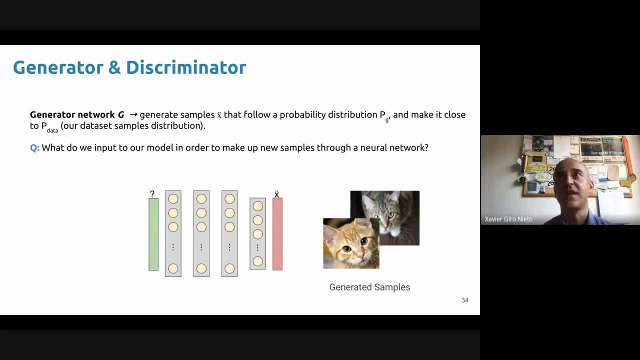 An example exactly with the same probability. So how can we change that? OK, great. So there's a lot of things. We have an answer, finally, on the chat. So the suggestion on the chat, which is a very good one, is like we could introduce some random white noise. 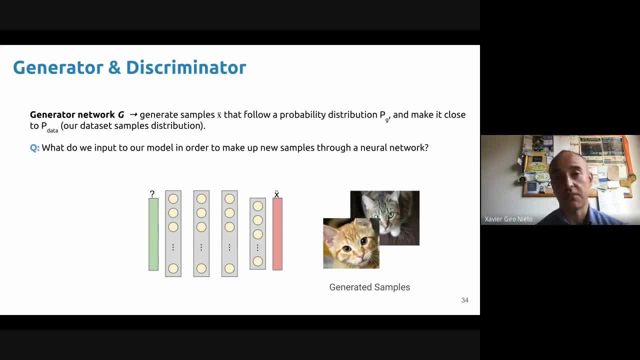 if you want, OK, great. So there's a lot of things. We have an answer, finally, on the chat. So the suggestion on the chat, which is a very good one, is like we could introduce some random white noise images, which is a good option. 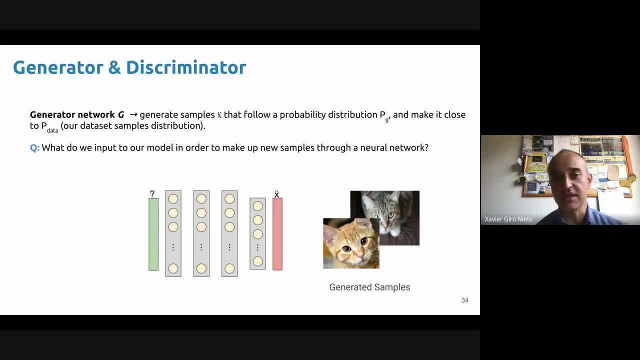 I don't think. probably we don't even need it to be images. I understand that it might be easier, maybe in terms of architecture, So maybe that makes it easier, But actually we don't even to have 2D, or yeah, I mean never mind, right. 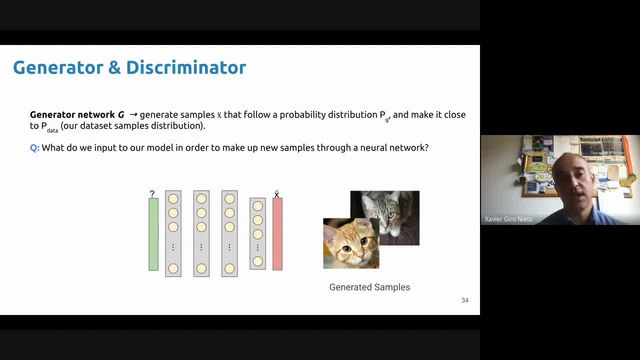 Just some random noise at the input, And so actually, what we're going to do, like on the baseline, baseline architecture, we'll be just sampling from some kind of Gaussian distribution. It could be 2D, it could be 1D, never mind. 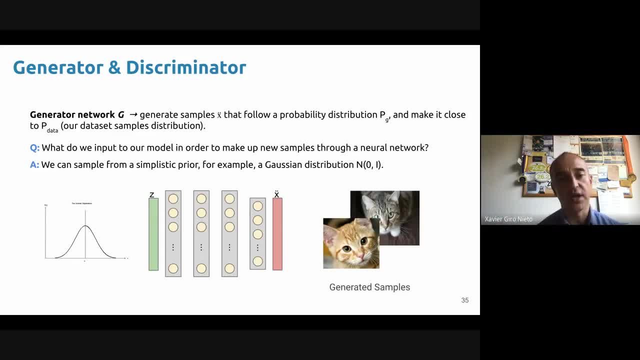 The architecture can take care later of making sure that the output is 2D and in color. This way we can assure that there's some stochasticity at the output. OK, do you have? do you know any other way? so that a network, so the same network. 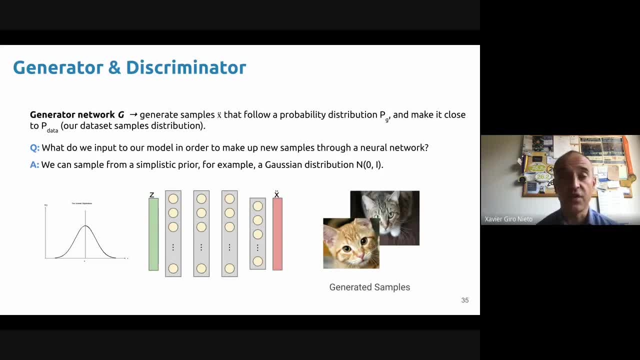 can have some diversity on the output. So one method that you have seen when training neural networks, which was very useful to avoid overfitting and that probably when we talk about it they said: use that only on training, never on the test. 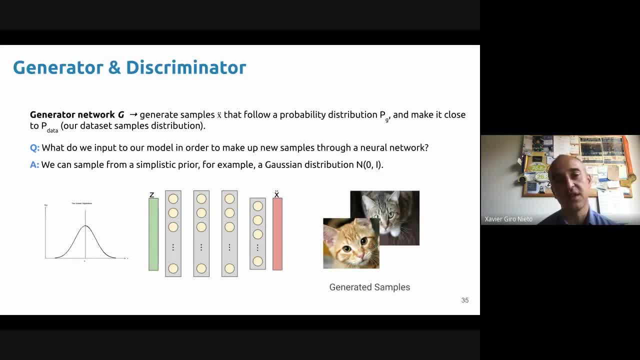 Yeah. so another option would be like dropout. So dropout means we kind of turn some neural networks, Yeah Neurons, off, And that's good for as a it's a good tool for regularizing and that's why we saw that. 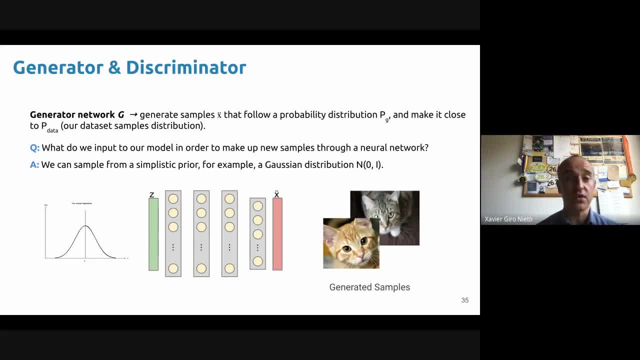 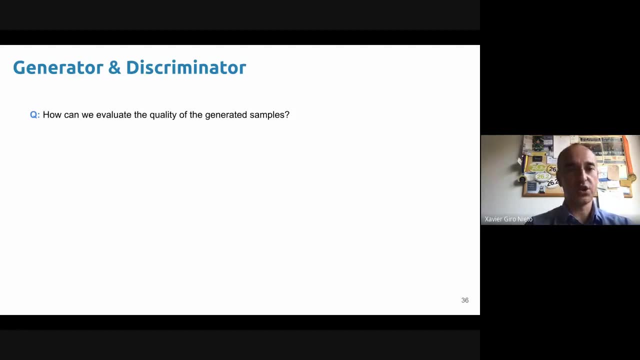 on the part on fighting overfitting, But you could also do that on inference time, and that's going to have like a similar behavior. It will also generate a diversity of outputs Then. so we have a generator that will generate samples, let's say, images of cats. 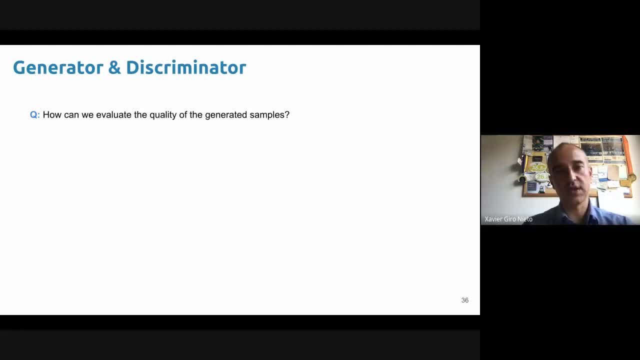 So who is going to decide if those images are good or bad? based on what I explained earlier, This is an easy question if you follow my explanation earlier. OK, So generator generates a diversity of images of cats. We have solved this. Now who is going to decide or assess if those images are good or not? that good. 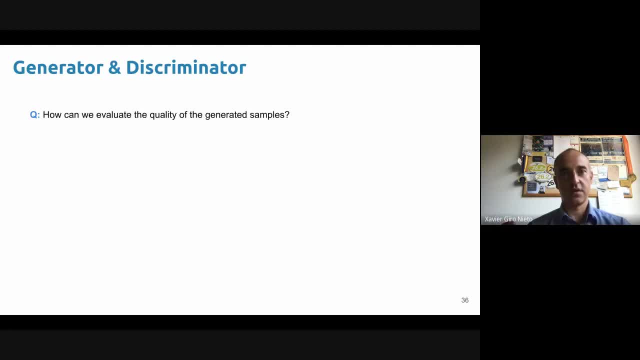 OK, OK, OK, OK, OK, OK. One clue for you is like. the answer is in the slides. We can make a discriminator. Thank you, Great, So yeah, So we have one generator Right now. today, I'll be talking about generative models. 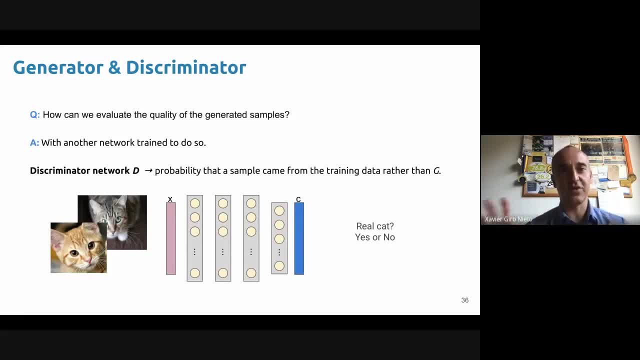 OK, I'm not. you see that I will not pay attention for discriminator much, although it's very useful for other applications. But today I'll focus on generative models. So kind of the discriminator has kind of a secondary role. OK. 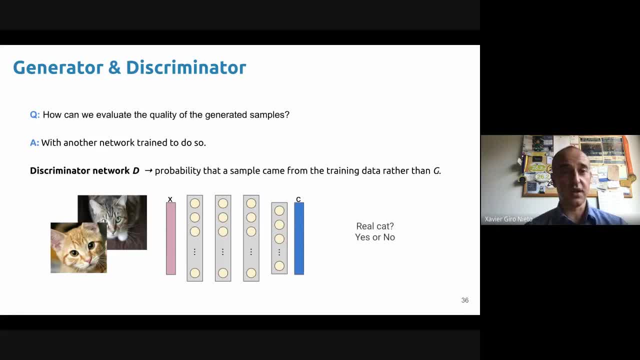 Because discriminator is going to guide the training of the generator. So we will have is at, we have another network that will be fed with images, But, whether real, whether synthetic, and the discriminator is going to be another neural network of can have, like any architecture. 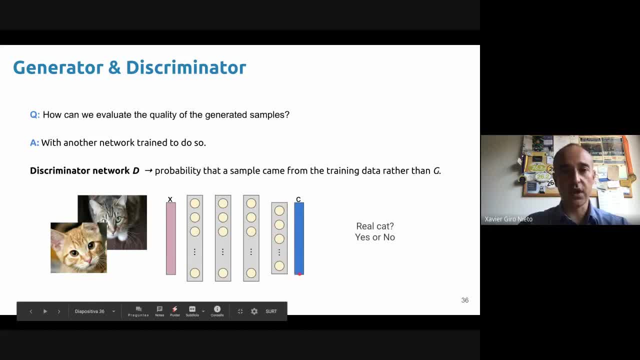 But at the end, basically, it will be classifying between real and synthetic images. So whether real or synthetic, OK, Whether the cat is real or not, That's going to be its role. So here you have a broad overview of the whole scheme. 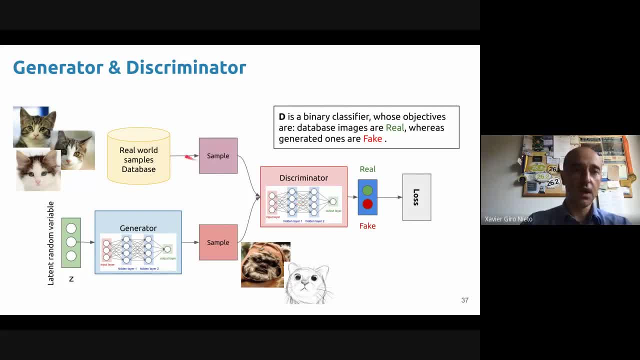 Let's look at it in detail. We have first, these are our real images, our real cats. It's our training data set. We have all samples database And from this branch. so this part is just sampling, So it means taking samples from the database. 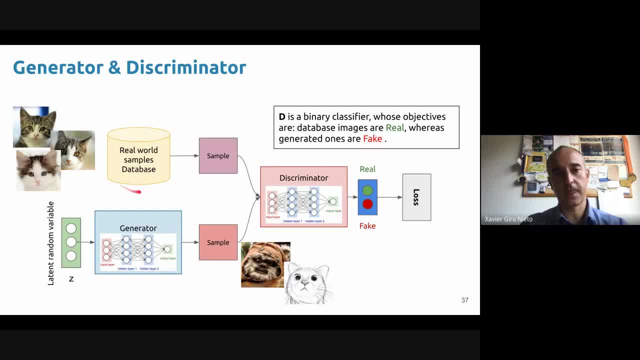 OK, From the training data set And we show real images here. And on the other branch we have a latent random variable- our noise that we mentioned. We feed that into the generator That's going to be again a neural network, whatever architecture, we don't pay attention. 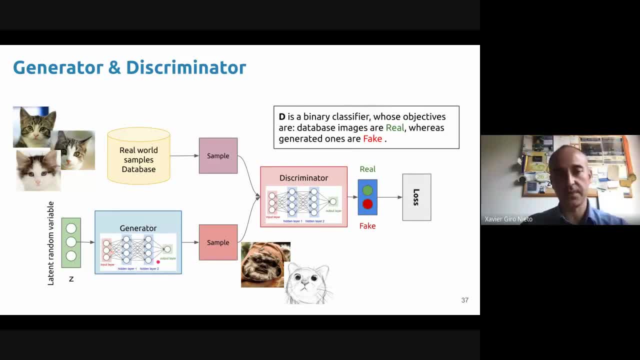 to the architecture. It just means this, just means whatever architecture, And this is going to generate images. OK, And maybe when it's learning, the cats that it's generating are not that realistic. maybe it kind of generates more like a new walk or a draft. 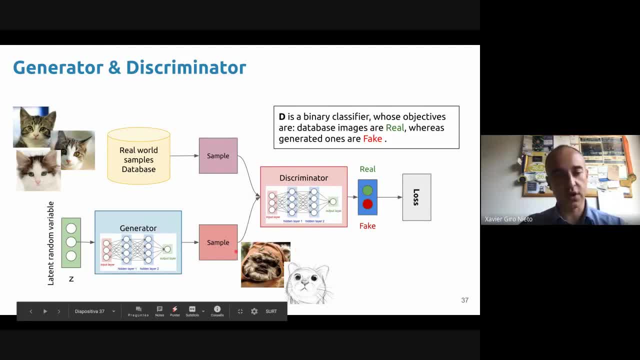 It's totally like, just to make an example, OK, that this will not happen, It will generate some blurry cats. But just to explain the story, let's say that generator must learn how to generate images of cats, Right, And then we have the discriminator. 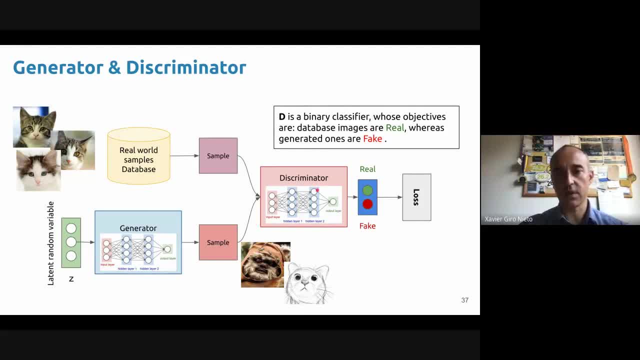 There will be another network again, never mind about the architecture, And this discriminator will be predicting whether the input- so sometimes- will feed real data, Sometimes will feed data OK, So if we have synthetic or fake data, the discriminator will need to decide the prediction. 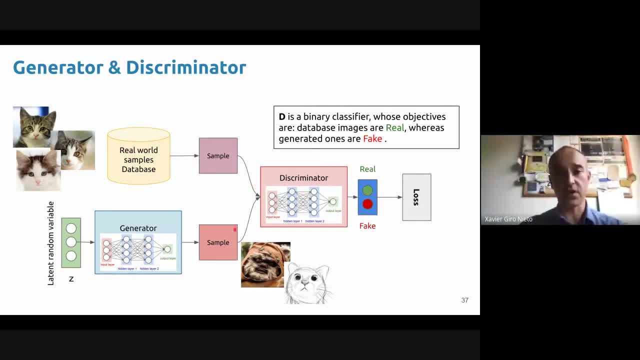 As we know, as we will always know, what are we showing to the discriminator. we will always know if the sample we feed here is real or it's fake. we will have kind of a ground truth label and we will compute a loss to compare the predictions of the discriminator with. 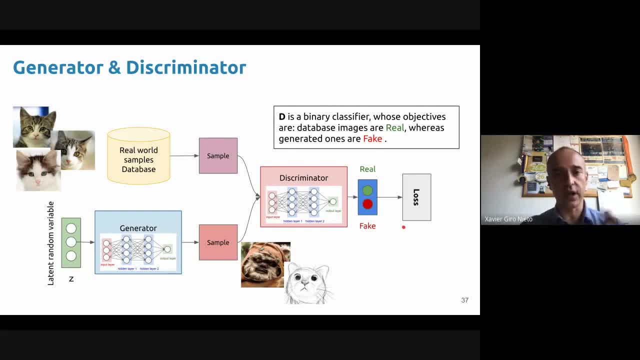 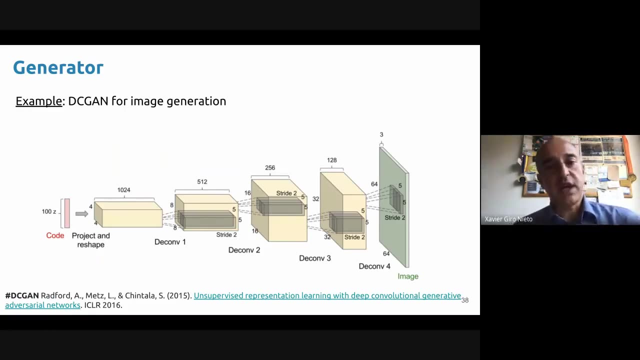 our label. OK, Let's say typically we can think about our label as a one-fault encoding, Let's say one-zero for real and zero-one for fake, for example. That could be an approach In those architectures as I mentioned. you could have like any architecture you can think. 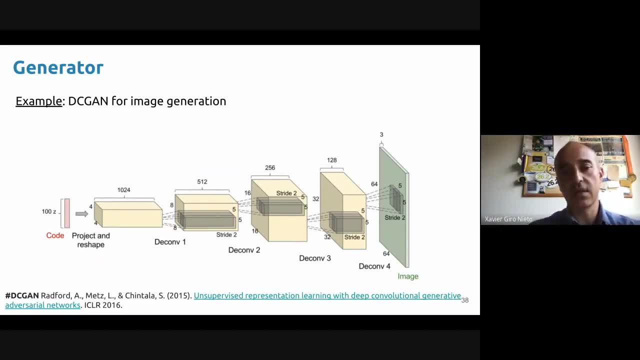 about. Just here as an example, you have one generator that was one of the first ones proposed to generate images, in which you fed at the input a code with a random variable of dimension 100. There were like some upsampling convolutions and at the end there was an image of in. 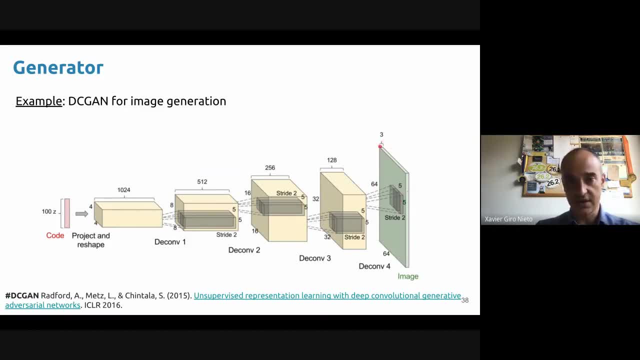 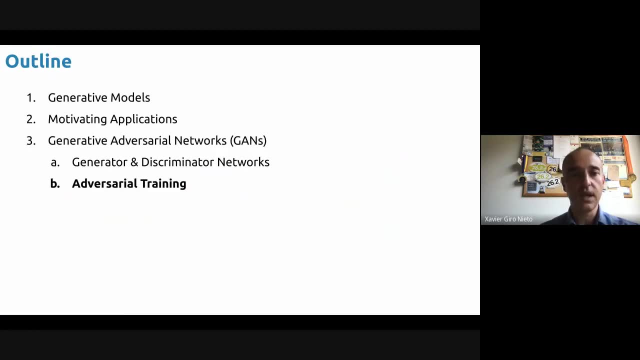 this case, 64 over 64, and the three RGB channels, which could be one of the first architectures used for image generation. Let's see about how to train these two networks. OK, Well, it's quite clear. We have two networks. 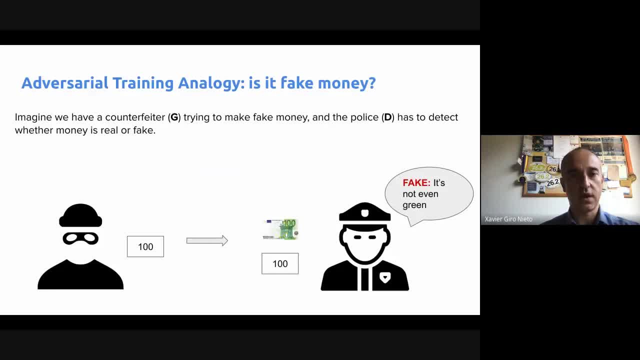 We know what we want them to do. Let's see exactly how we train them. So I'll start with an analogy. So this training will be very iterative, will be kind of a trial and error, especially for the generator. Let's imagine that we have an analogy, which is we have a counterfighter. 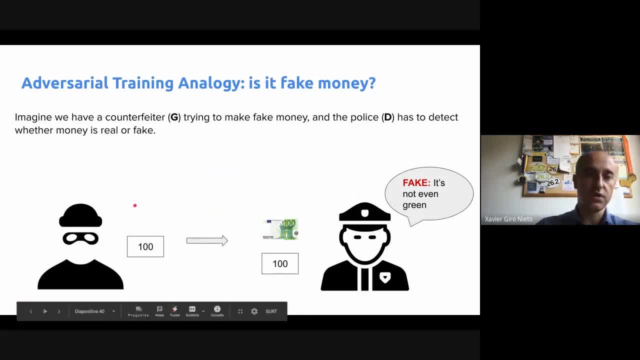 So this counterfighter, its goal is to, he wants to create, generate fake money, OK. And then there's the law enforcer or police that will try to stop the counterfighter. to generate fake money, To fool the generator, To fool its citizens, the rest of the citizenships, OK. 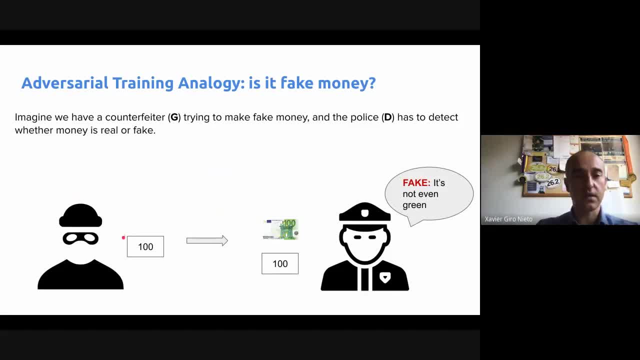 So let's at the beginning. the counterfighter is really bad at generating fake money And he shows this white rectangle to the with a 100 written to the police. The police compares the real nodes with the fake ones and says that's very easy, OK. 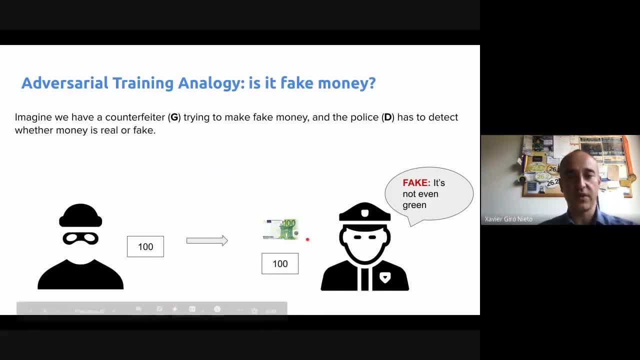 And actually it kind of gives tips to the counterfighter, like, OK, it's not, it's so easy, right? It's not even green right. So with this information, the counterfighter will learn to improve its output, its outcome. 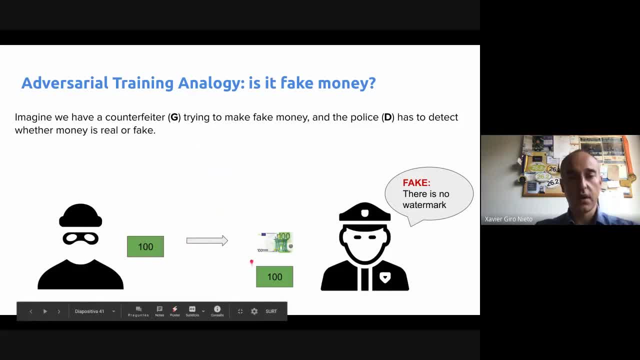 So now the node it's green, But still the police says: oh, but there's not even a watermark, so it doesn't have this nice logo here. And then the counterfighter adds a watermark, and now the police says: OK, the watermark. 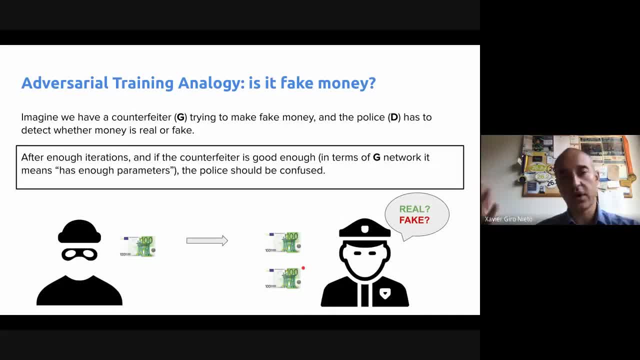 should be rounded, and so on, and so on, and so on. And at some point, At some point, if we manage to train our networks, the counterfighter will be able to generate banknotes which are as realistic as the real ones, and the policeman will be. 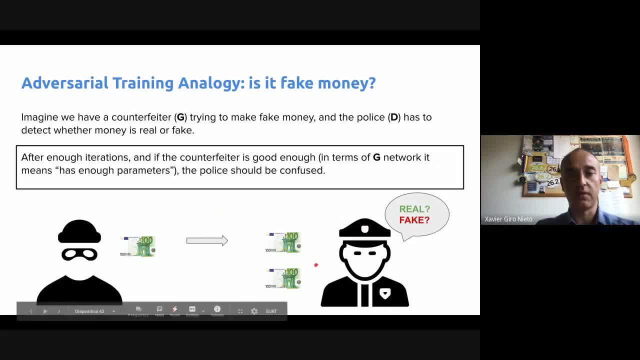 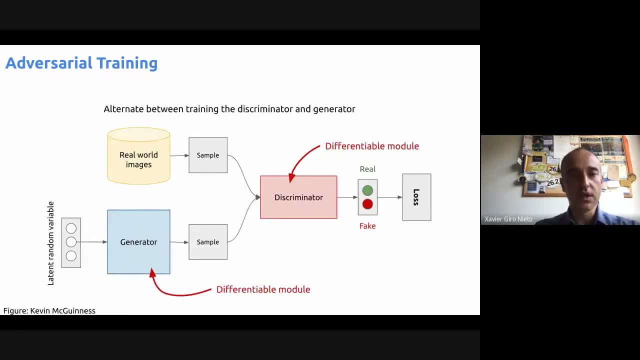 really hesitating between real or fake. So when it predicts real or fake, the chances that it gets it right it's going to be like totally random. let's say 0.5.. So if we look at this example with the figure that we showed earlier, 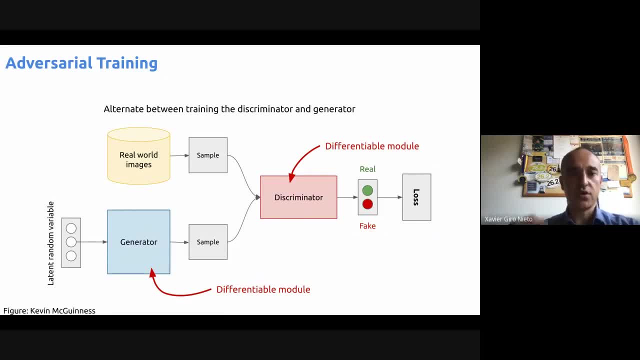 What we have now are two models which are differentials. so these are our neural networks, for which we need to estimate the parameters. We have the discriminator and the generator, And they are aiming at different, contradictory goals. So how are we going to do the training? 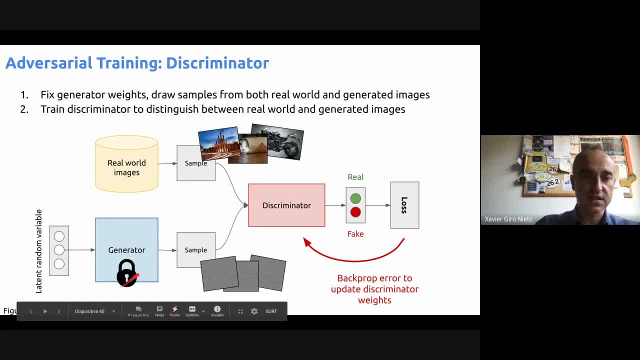 So first, what we do is to fix the weights of the generator. Look here I fixed the weights of the generator. OK, That's this block. That's what it means. What we do now is so, whatever weights that the generator has, we start fitting with sampling. 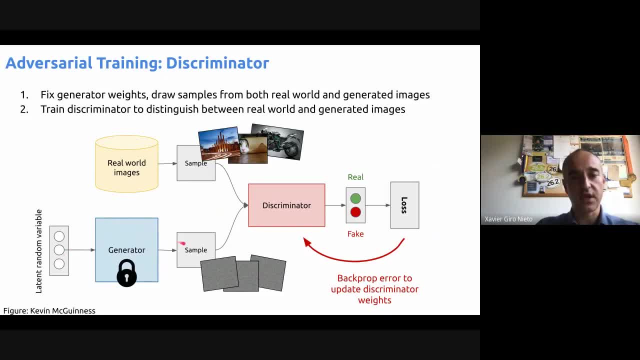 from our latent variable, our noise, let's say. it's still generating samples At this point, at the beginning of the training. it's really bad. it's just generating random images, While on the other hand, we have real-world images like these ones that we show to the 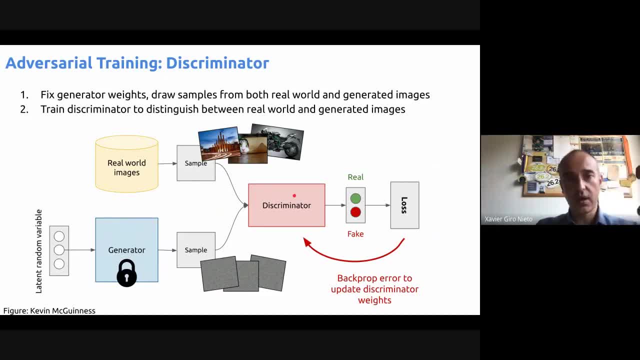 discriminator. And now, at this point, what we'll be doing is training the discriminator, So we'll be just computing the loss for these images, for these other images, see the deletion of the discriminator, and then back-propagate radians to the discriminator and the parameters. 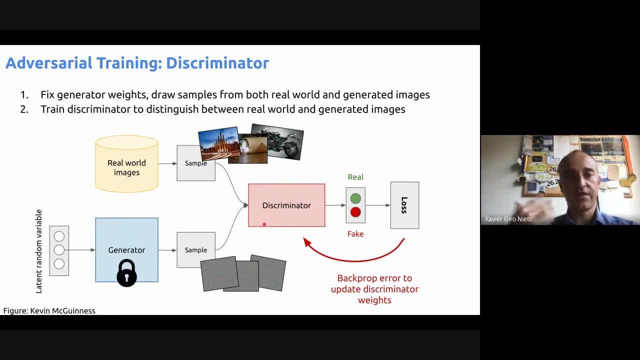 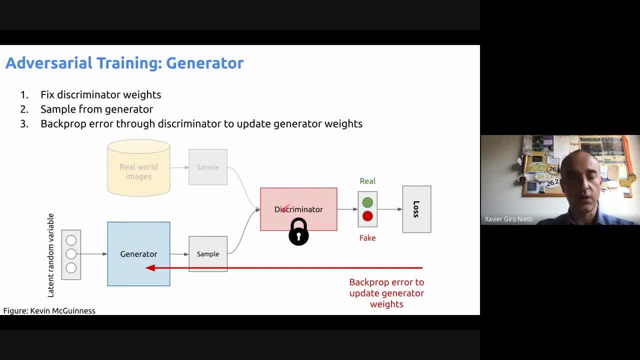 And we do that for a few iterations. After a few iterations we change the role. Now we lock the weights of the discriminator. They will not be changing, They are fixed. We unlock the weights and parameters for the generator. We fit the random variable. 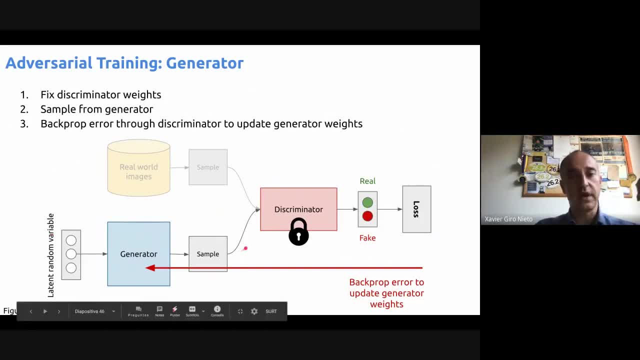 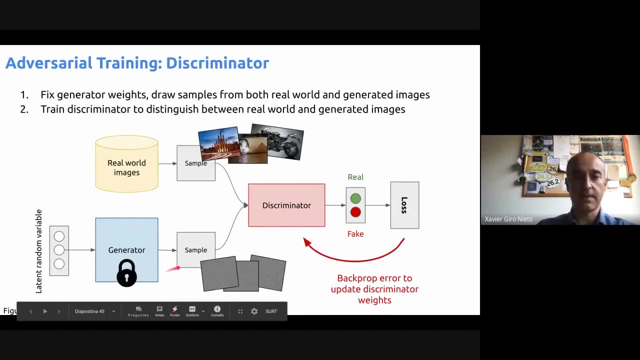 We generate fake samples, The discriminator does the predictions And what we want now is just the opposite of in the previous case. If earlier, when we were showing fake examples for the discriminator, we had a loss, We had a loss. that was kind of encouraging that these images would be labeled as fake. 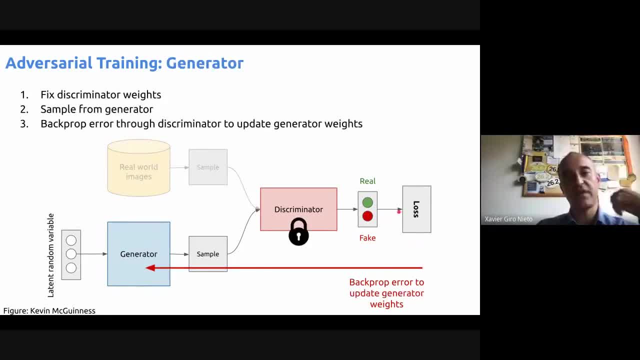 Now we totally change our loss And now we have a loss that will encourage that these sorry that the images that come sampled as synthetic, they are labeled as real Because now we are training the generator. At this point we don't care about the discriminator. 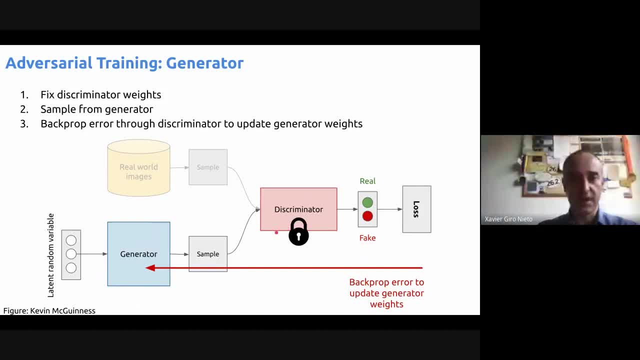 We want the discriminator to do a very bad job. We want to fool the discriminator, So now we have a loss. We have a loss, We change the labels And we want the generator to fool the discriminator. So we want that these images that we sample, they are labeled as real. 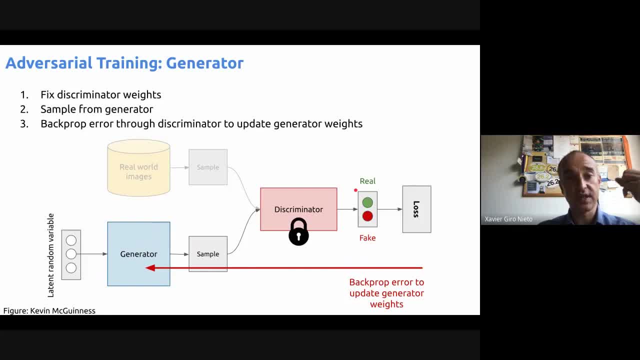 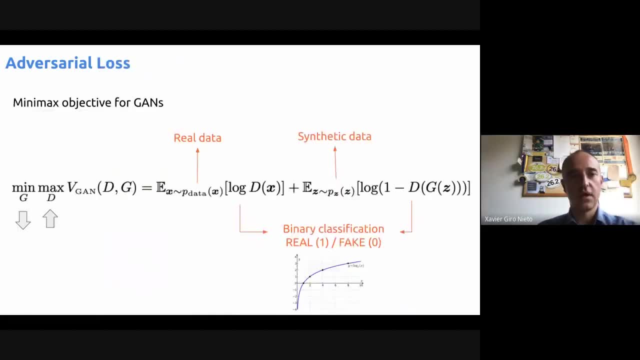 Okay, You need to do this in the lab this week. If you look at the expression of this process, that's what's called the mini-match objective for a GAN And I'll show you. I'll explain it to you. I think if you understand the idea, it's quite easy and it might be intimidating at first. 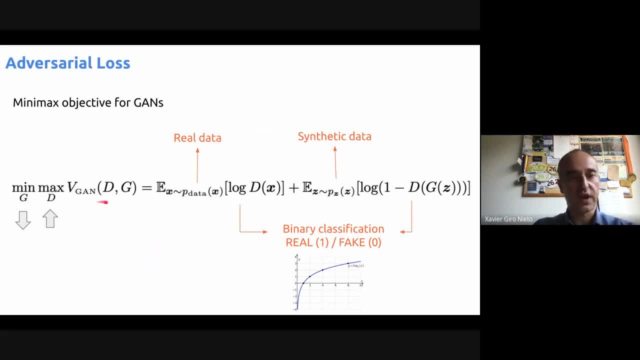 We have, let's say, a value function or a loss function for GANs And we have first look at there like two different goals, right? So the generator will try to minimize this expression and the discriminator will try to maximize the expression. 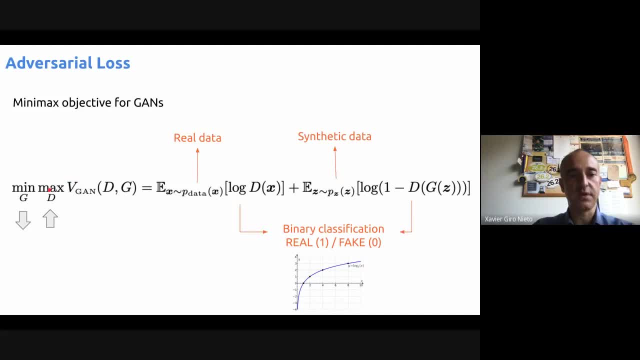 So let's see what they're trying to do. Let's see what they're trying to do. Let's focus on the discriminator first. So discriminator when it looks when we are sampling data from the real data distribution. so data it means like the real distribution. 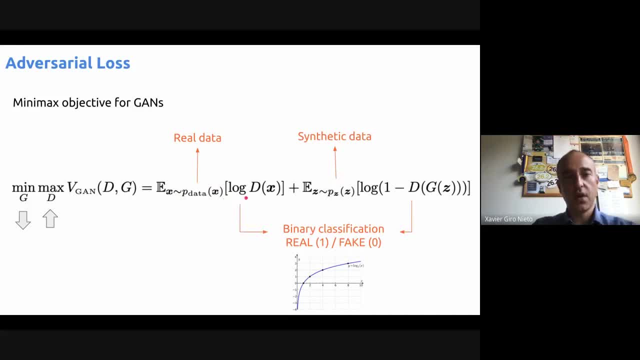 So that's real data. The discriminator will try to maximize this part, So it will try that the output of discriminator is high. Okay, Actually there's a log, but the log is an increasing function. okay, So we want it to be large. 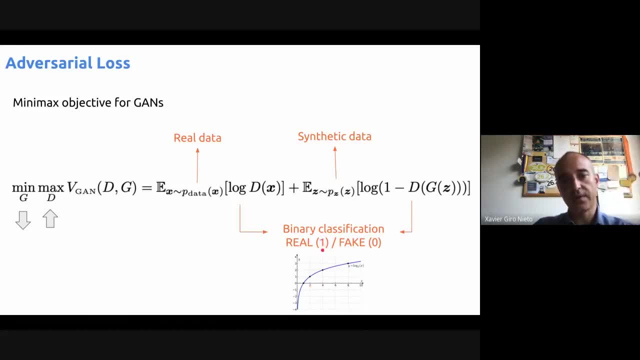 So we'll try that the prediction one is the correct one, So we'll try to predict a one. On the other hand, when we have synthetic data, it's going to be just the opposite, right: The discriminator. So on the discriminator. we have now for the discriminator. it has one minus and that's. 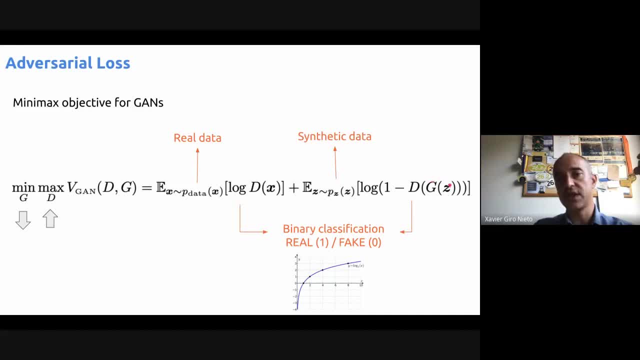 the g of z, So the z is the noise, So g of z is the image that was generated synthetically. So d of g of z, this g of z is the synthetic image, while x is the real image. So when we are fed discriminator with a synthetic image, it will discriminator, will try to. 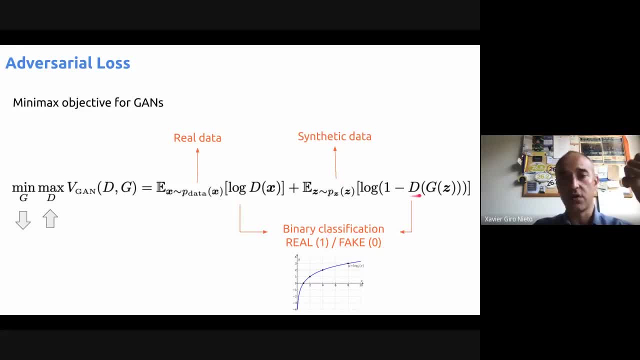 make it small. That's why you have like a one minus. So earlier we had the discriminator like pushing up towards the loss value. Now, as we have a one minus, it's just the opposite direction. On the other hand, if we focus in this term, if we now, we forget about the discriminator. 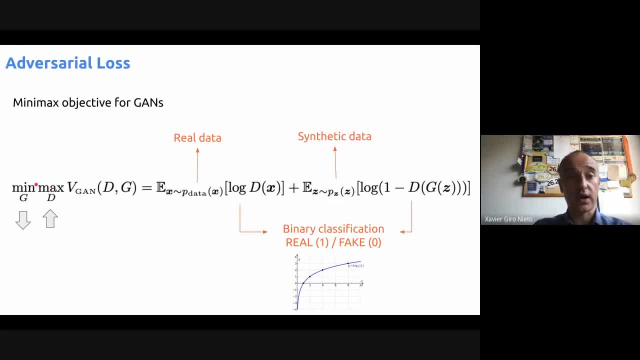 and we focus on the generator. it will be one, actually just the opposite of discriminator. So if discriminator wanted this term to be small, Okay, Okay, Okay, Okay. So if he wanted this term to be large, okay, the generator will try just the opposite to. 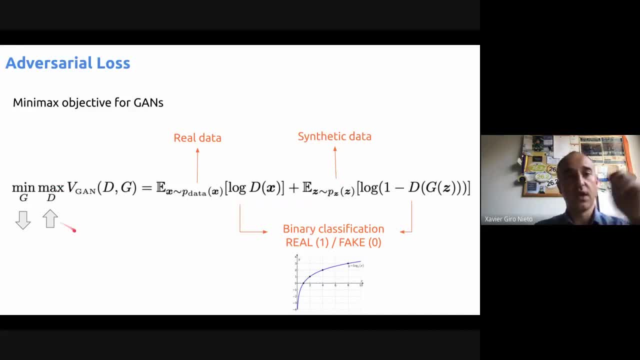 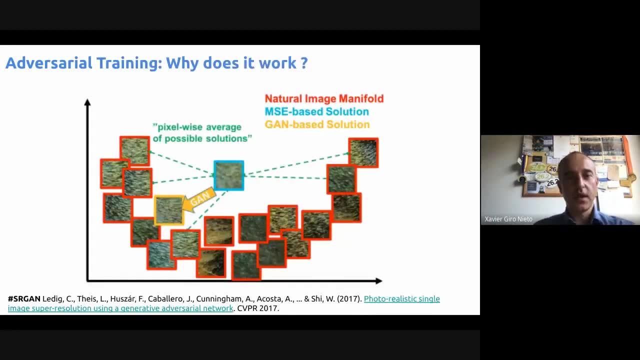 make it small. So we're trying to minimize. Okay, So that will be the mathematical expression for GGAN- In a qualitative way. what's happening here and why adversarial loss is held, let's say, compared with a mean square error solution is that GANs kind of force. 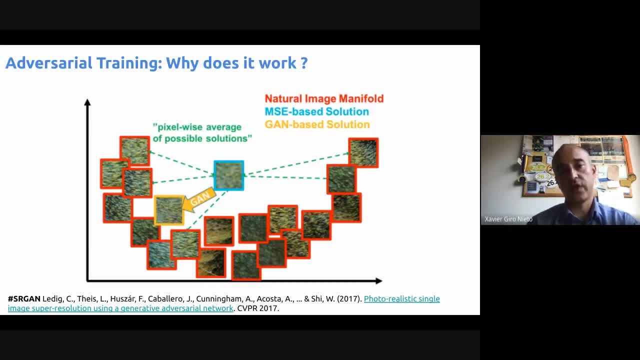 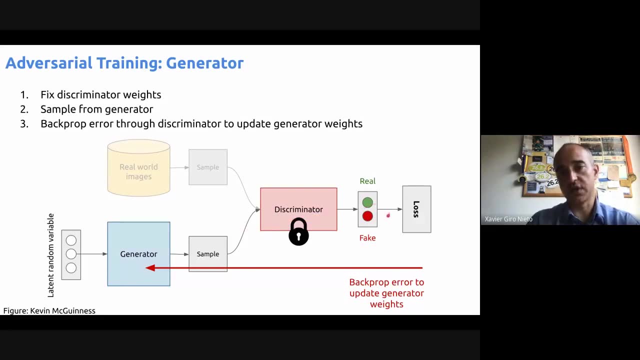 The networks to take a decision. So if you try the network with only the mean square error, that's something that we could do. We could when we know that when we are predicting, like this, output one or zero, okay, we could just have a mean square error here to predict, to compare as a loss function. 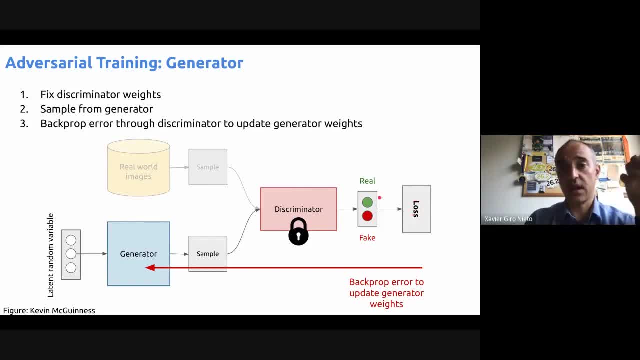 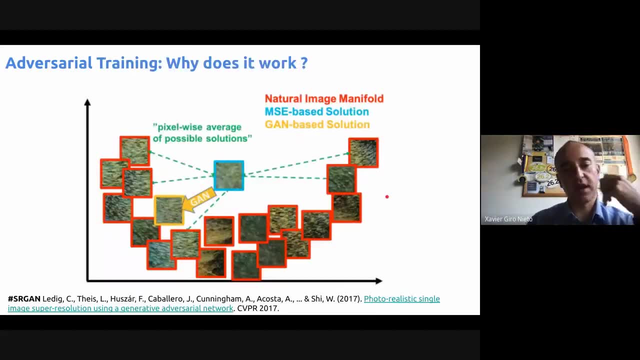 Okay, If we take the loss function as a mean square. Okay, As a mean square area. error. what the networks will try to do, it's kind of not take any hard decision Like you will try to minimize the loss, like on average. 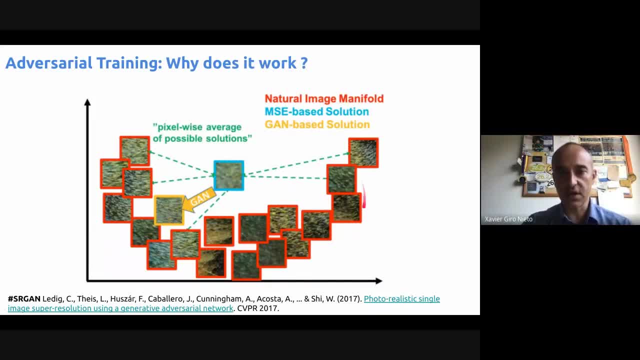 So when we let's say that you need to sample images, crops like this and all of them, they kind of look they are. these are all like real crops. Okay, Whatever I said, that nobody's. what is that? 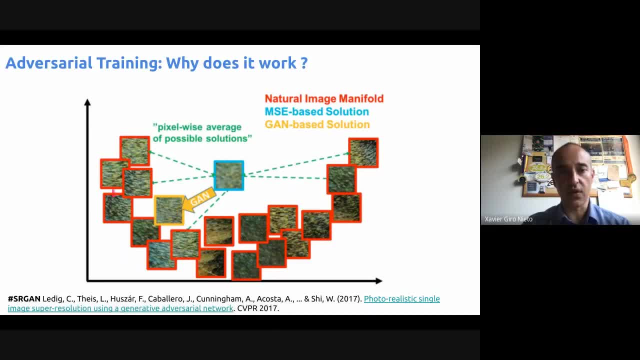 But if that's your training data, Okay. So in red are our training crops and we use a mean square error based solution, the mean square error based solution. So with no adversarial loss, it will jam to generate samples. They are that, they are kind of the average, because in the end the average solution. 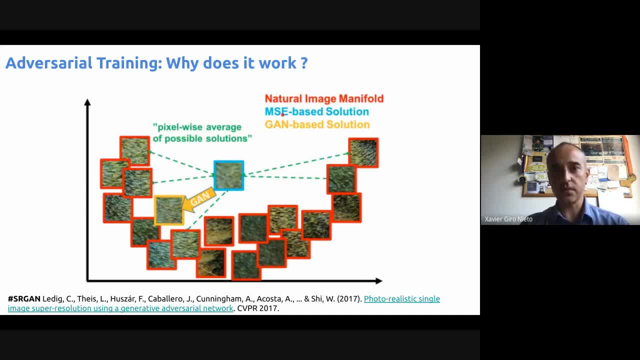 that's what minimizes the mean square error. And then, if you try that, you'll end up with samples that don't look realistic, but they'll kind of look blurry, Okay. So on the other hand, if we try with a GAN loss, we'll generate samples that are much 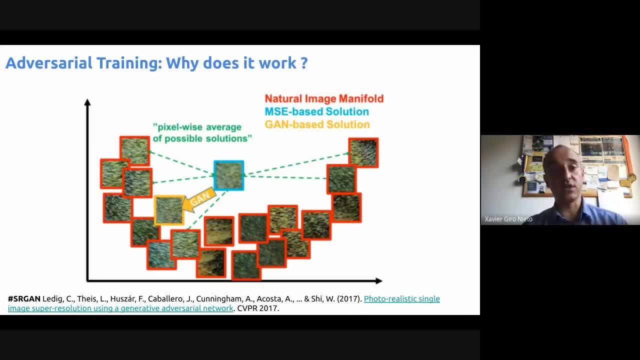 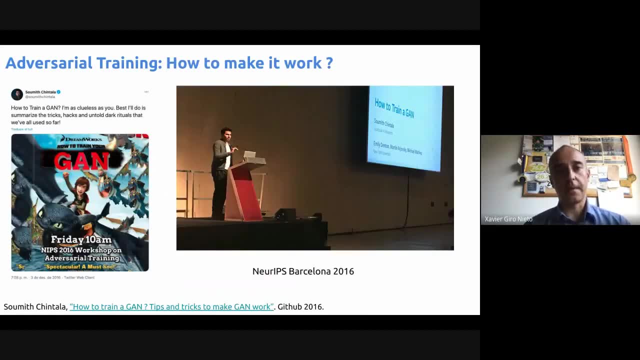 more realistic. That's what you observe And actually in many cases what you do is we combine GAN, adversarial loss, with other perceptual loss. Then if you want to train a GAN, there are many tricks. they are very stable to train. 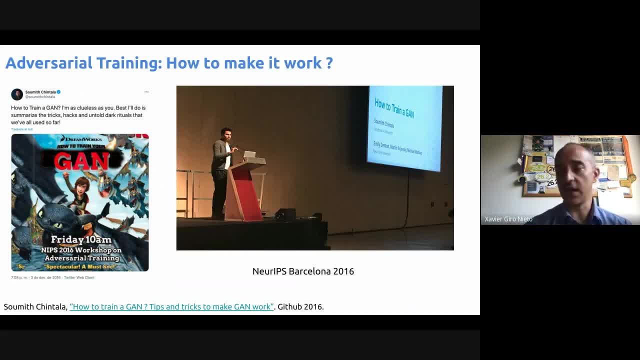 So I strongly suggest that you look at this tutorial, that from Sumit Chintala on how to train a GAN. Okay, Actually, it was presented in Barcelona, It was the year of the GANs and there was so much hype on this and they were, and he. 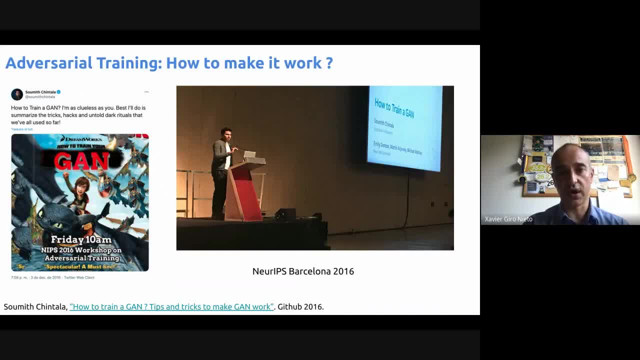 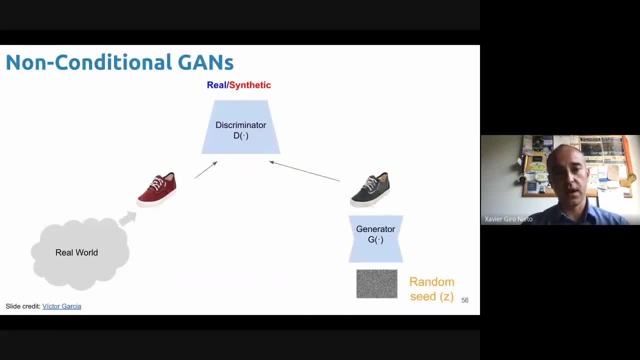 gave a very nice tutorial, actually, like other speakers, for sure, for sure told there. Then there's a variation of GAN in which: what if, instead of just having a random seed for the generator, why don't we condition the generator? 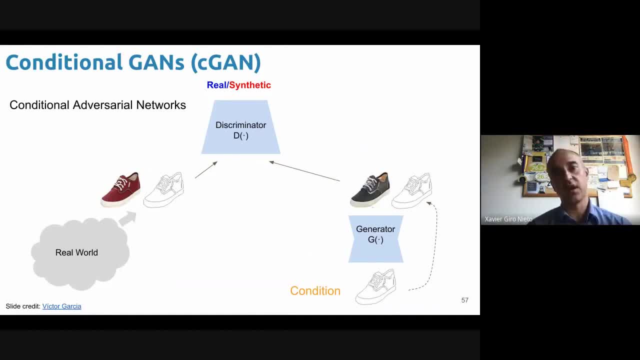 So we kind of now we want to have some control, don't just feed noise into the network, But let's try to control what's being generated. So what we could do is I imagine that we have like some condition. let's say a sketch. 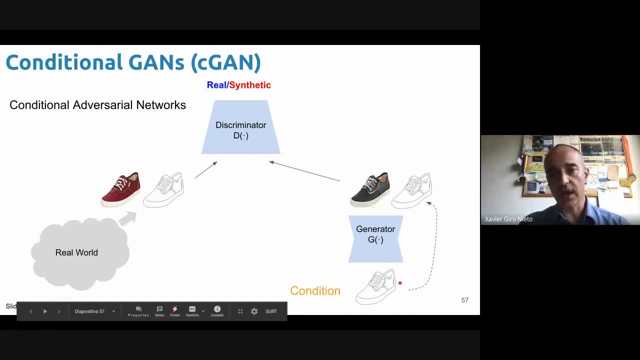 of a sneaker or a shoe, And then we would like to have, it's like, to condition the generator so that the output sample it's it should match to this condition. So this, in this case of this sketch, That's what it's called. 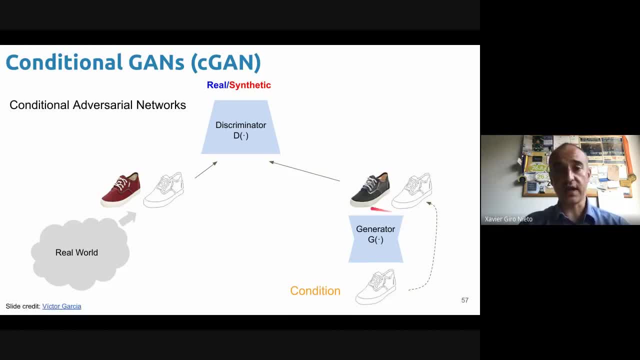 Okay, So we have conditional GANs or C-GANs, And if we train with that, we need these pairs for both the real training data and the generator, Because for the discriminator we will not only be showing the real or genetic sample. 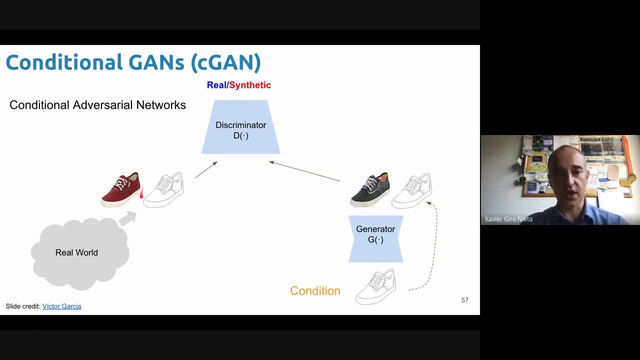 but we will also show to the discriminator the conditioning scheme, the conditioning data we have, And the discriminator will also evaluate, actually, if the match is correct, if even maybe you have a sample that looks very, very original But doesn't match the condition. 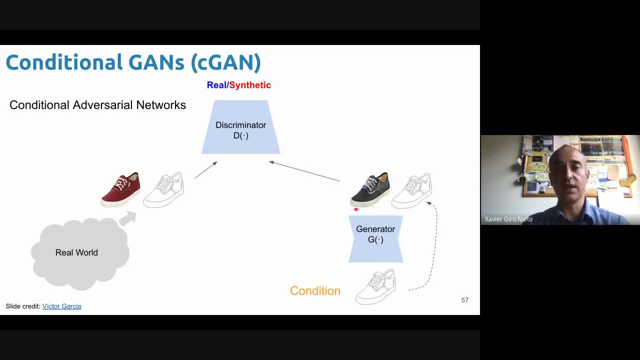 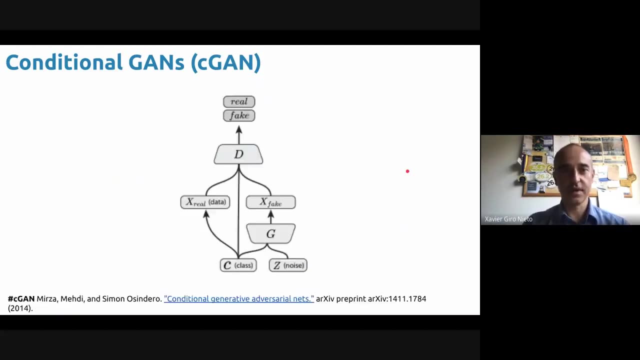 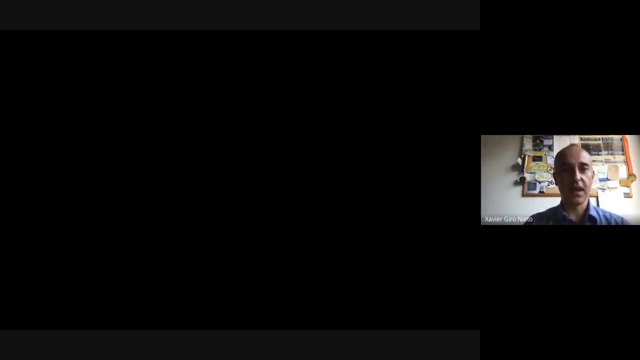 And the discriminator will also penalize that. So this way, the generator will will not only to generate realistic samples, realistic shoes designs, but also the shoe design that matches the condition. This is a scheme that I showed that could be like the original one from Misa and Osindeyo. 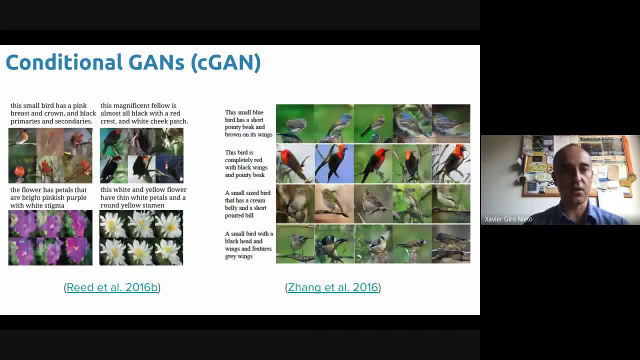 And that's kind of some of the words that you may have seen Or that you can do, In this case you. these are all images of birds and flowers that were generated with a description, a textual description of the bird or flower. 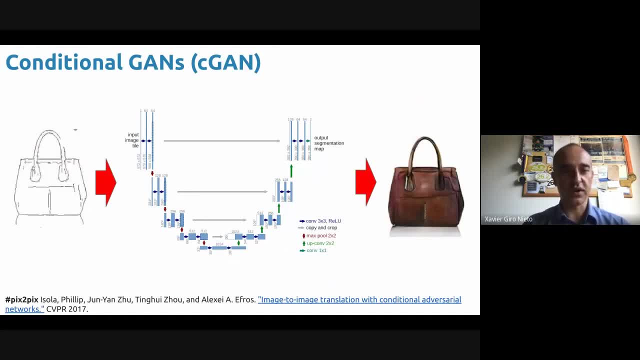 One of the most celebrated application of this approach, it's what's called the Pics to Pics model, in which, as I mentioned you, we can kind of do something called image translation somehow, And in this case what you show in the picture. 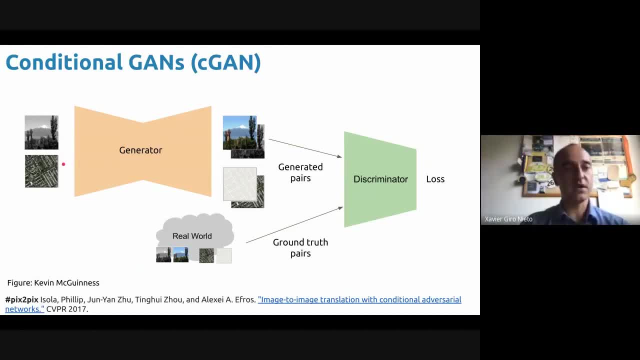 Okay, So the generator are pairs of. sorry, you have a light conditioning image And you have the generated one, So you have a new version of the image And then for training you need to have pairs of what. whatever transformation you are trying, 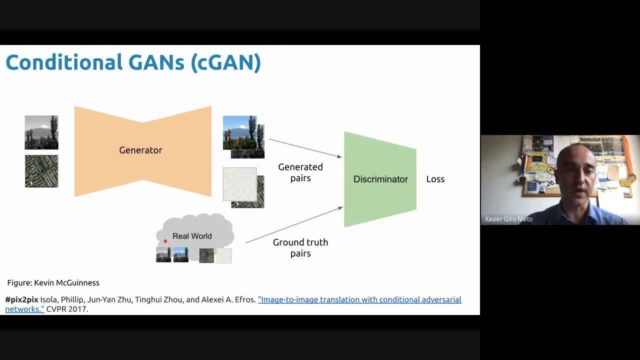 to do Whatever image translation you want to do. If you go want to go from grayscale to color, you need to have a data set of images that go from grayscale to color. If you want to draw the map of some some, 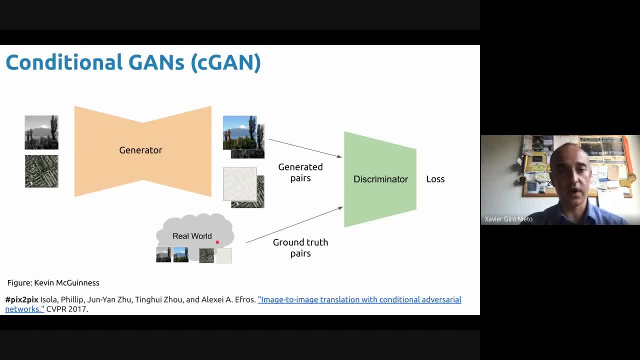 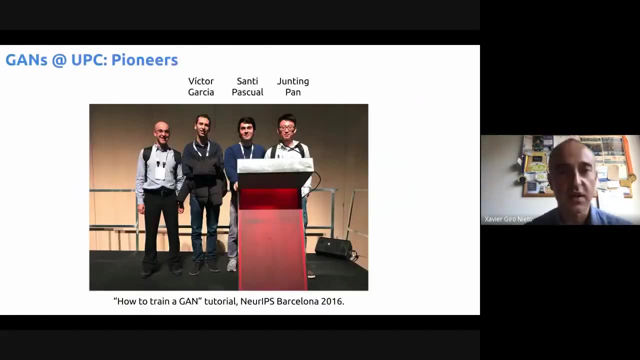 All right. So in this urban area you need the data set of real images and real maps, And if you do that, you are able to actually train models to translate images in different modalities. Okay, Just to finish, I'll just briefly present some words that have been developed at UBC. 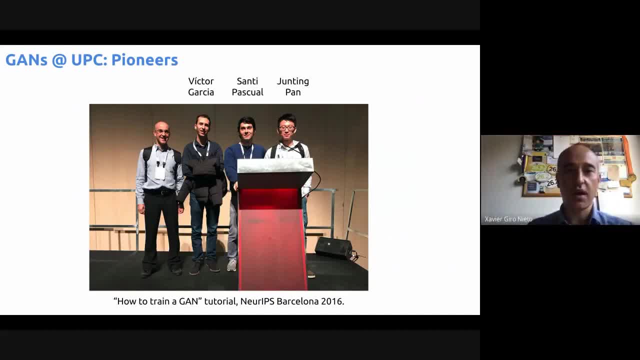 that I think it's interesting that you are aware of First in Jersey, like Victor Garcia, Sandy Pasquale and Junting Pan, which as far as I know they were pioneers at UBC in applying GANs. So 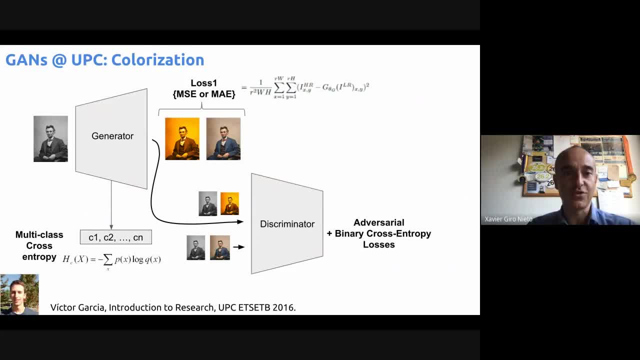 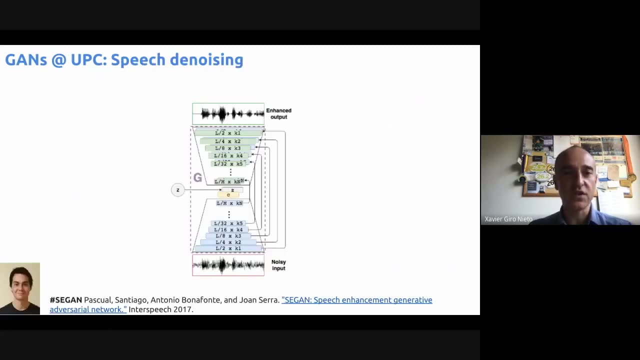 Victor was working on- actually with a Pics2Pics in parallel to the real Pics2Pics- in trying to solve chlorization, but they managed to do it much better and faster than we did, but still a very interesting work. Then Sandy Pasquale was one of the first authors that applied GANs into speech with a model. 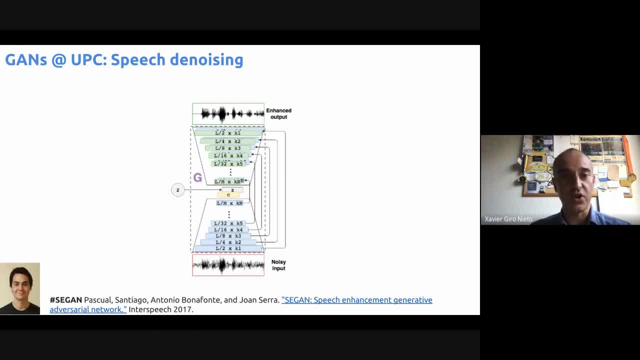 called SEGAN that was used to for speech de-noising, so to clean the noise from speech, And Junting was one of the first authors that applied GANs into speech with a model called SEGAN that was used to for speech denoising, so to clean the noise from speech and Junting. 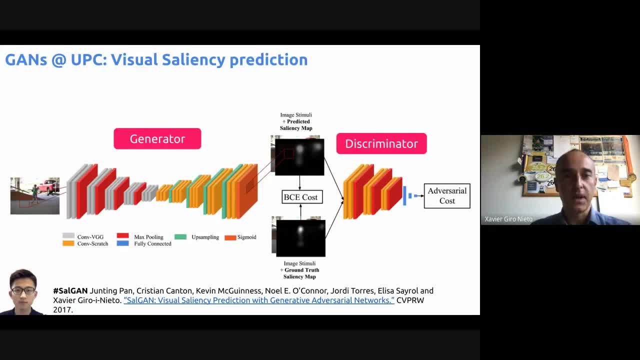 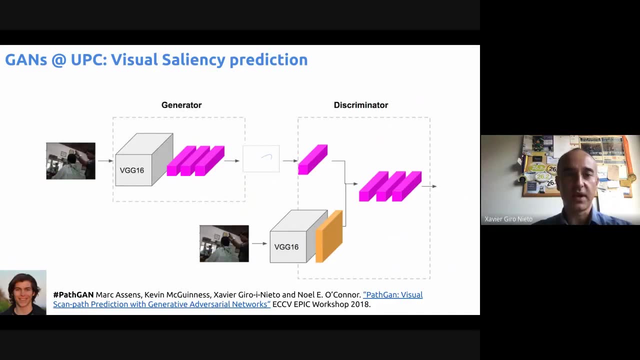 Jun-Chin used it to improve a model for what's called visual saliency prediction, which is like: given an image, try to predict the fixation points of the human case. Later, actually, there was a continuation by another student. Marker sensed that not only was he predicting the map, 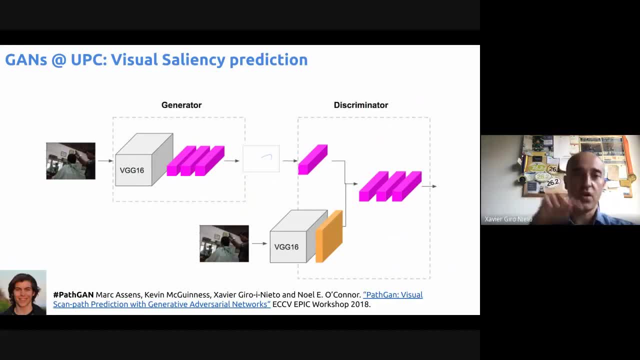 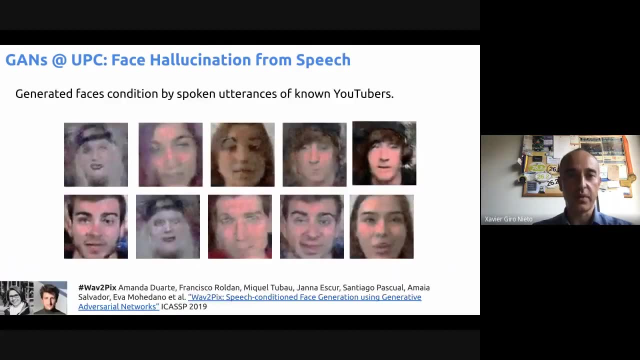 but he was also predicting the realistic path over the image of the eye case. And actually we won a couple of awards with this work, More recently with our PhD student, Amanda Duarte, and a master's student at that time, Miguel Tubaba and Kandisco Roldán. 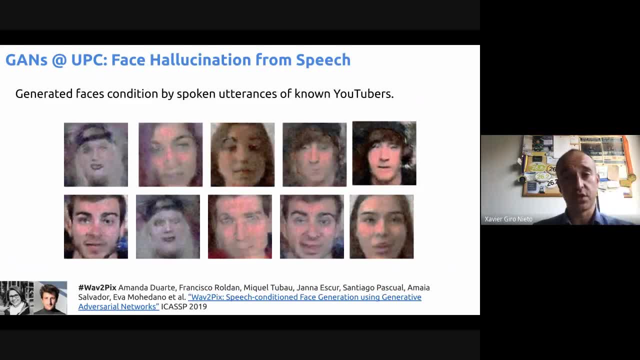 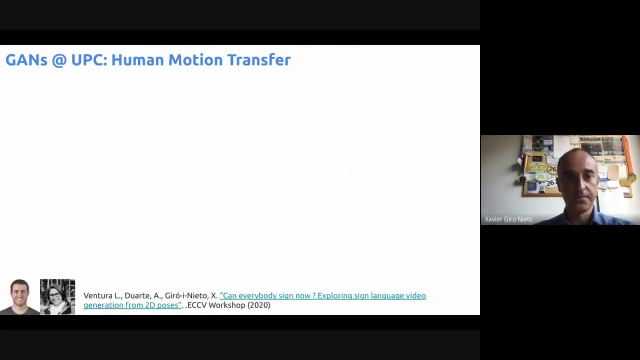 we managed to generate images of YouTubers based on the speech. So actually, we built a data set of pairs of frames- the faces from YouTubers and utterances from their speech- And we conditioned the generation of faces with the speech we extracted. 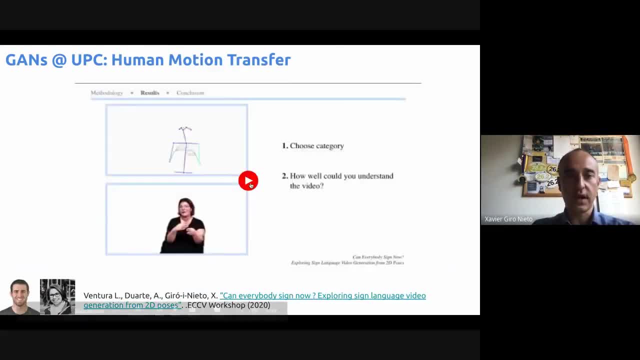 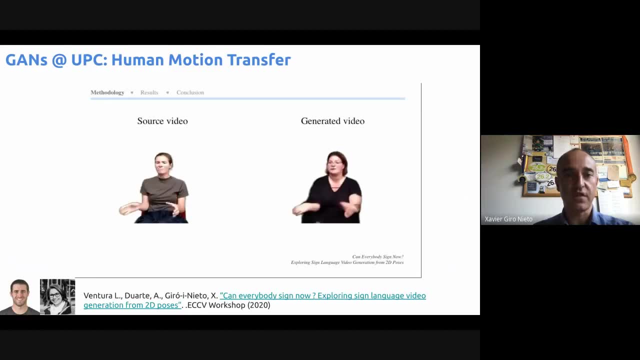 More recently even, we have this work from Lucas Ventura and Amalia Amanda Duarte, in which what we do, like this human transfer that I showed earlier for slang words. as you can see on the left, we have a source video that is transferred. 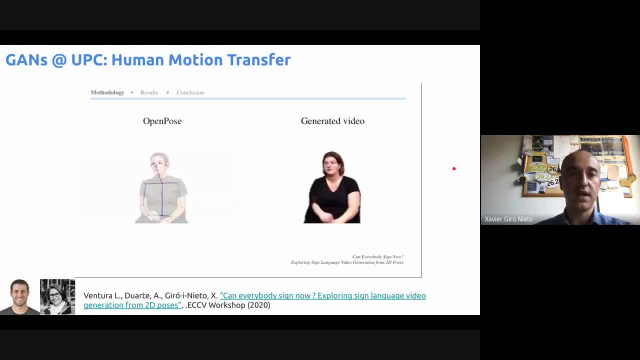 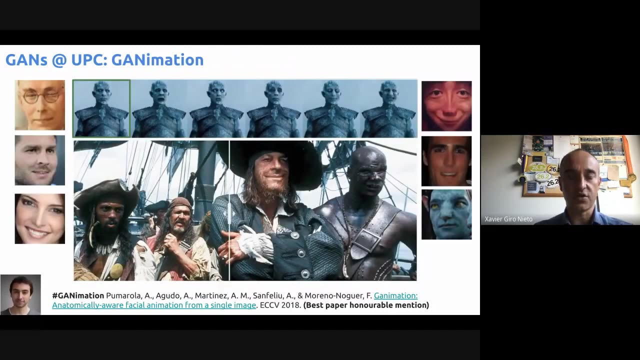 to the lady on the left, And we are working on this again, as in the first word that I showed you, that's based on first extracting joints from the body. From another group, from the Institute of Robotics, Industrial Robotics, IRI, there's 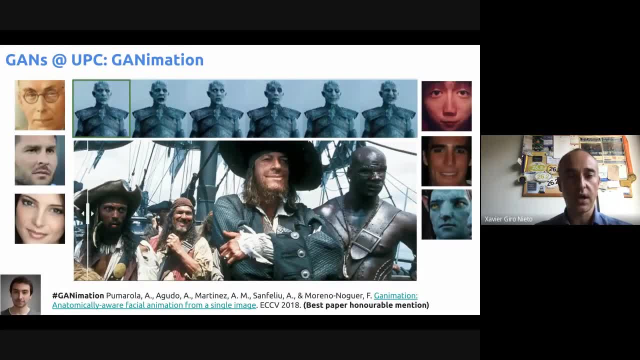 this word that's very well known- called Ganimation, in which Albert Pumarola and the rest of the team. they managed to change the facial expressions in a continuous manner. This work, actually it was awarded two years ago in ECCB. 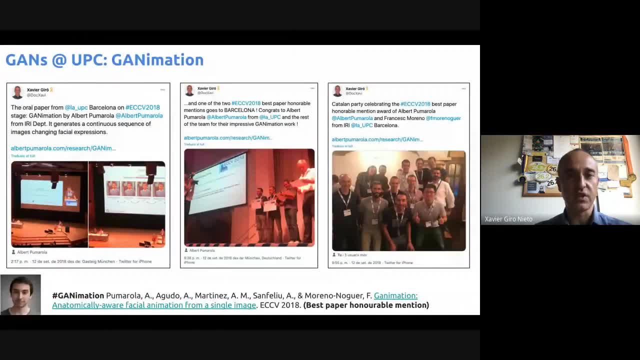 That's one of these very big conferences in artificial intelligence And he received the paper honorable mention. Unfortunately it was not in the front cover of our media but it is now. You can see it in the slides and you can be aware. 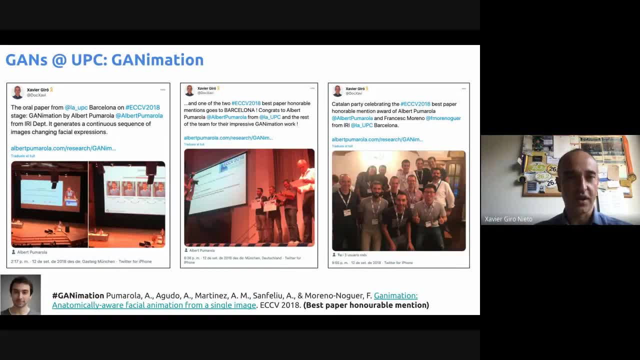 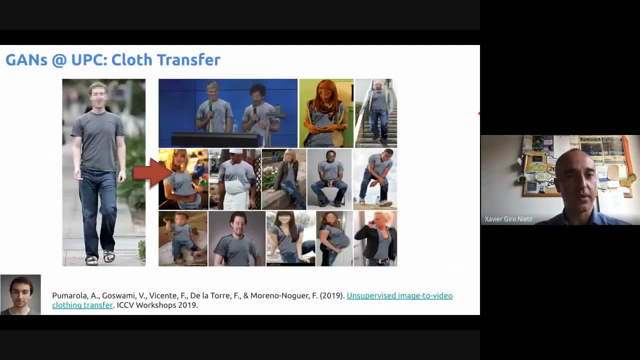 If you can see Albert or Frances, you can congratulate him for the excellent work. I think, Yeah, and more recently also, Albert had this work last year in which he was transferring clothes from one person to another. So you can see, here you have the popular shirt. 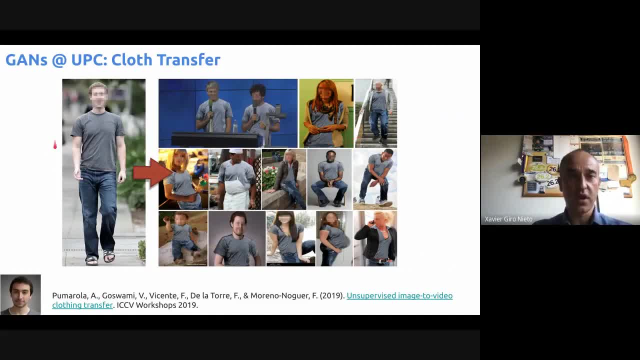 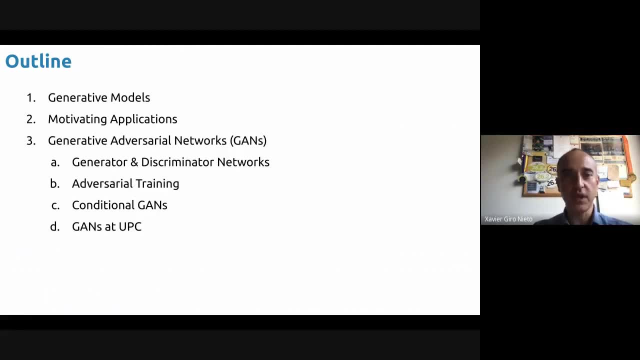 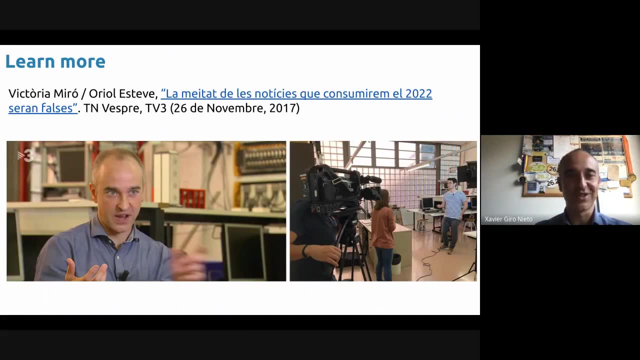 from. So actually he was doing an internship at Facebook and he kind of made everybody wear the same t-shirt, as you can see. So that will be it for today, If you want to know more here. Just like a very basic talk or very short report. 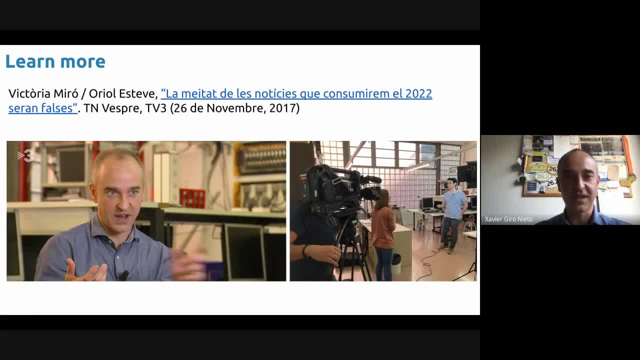 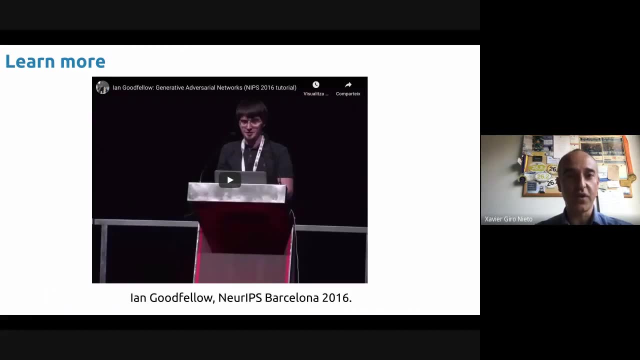 that where Santi and me talked about guns to the Catalan TV a few years ago when they were very concerned about deep fakes, because that's the kind of technology that powers deep fakes- And maybe much more interesting. you can watch a tutorial from Ian Goodfellow here.